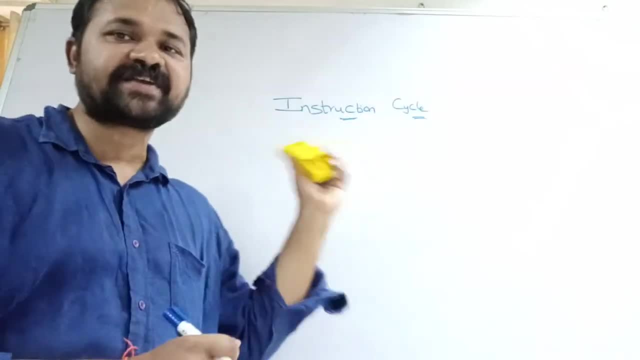 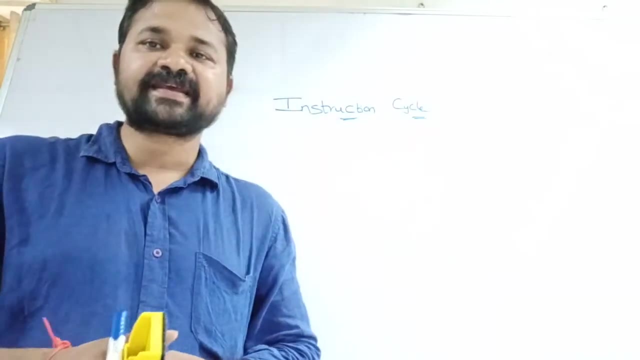 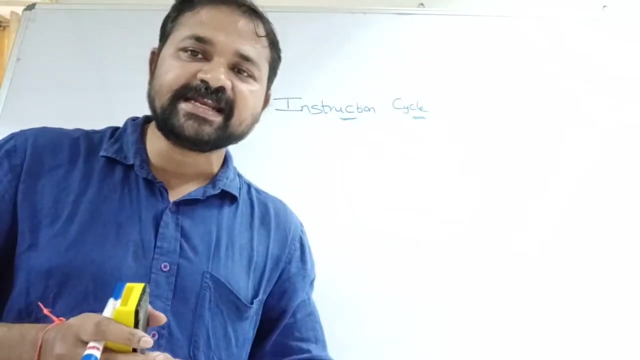 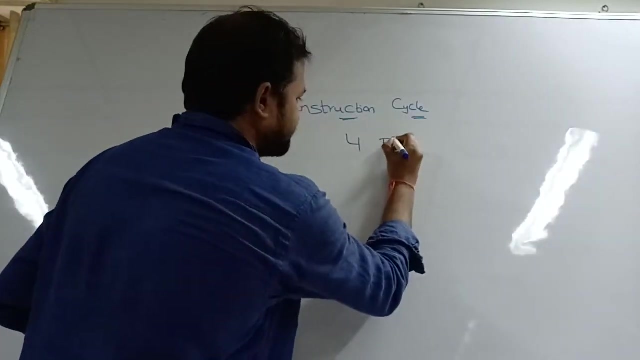 In this video we are going to discuss about instruction cycle. We know that every program is a collection of instructions, where each instruction is executed with the help of instruction cycle. Instruction cycle is mainly divided into four pages, So instruction cycle mainly contains four pages. Let's see those four pages one by one. 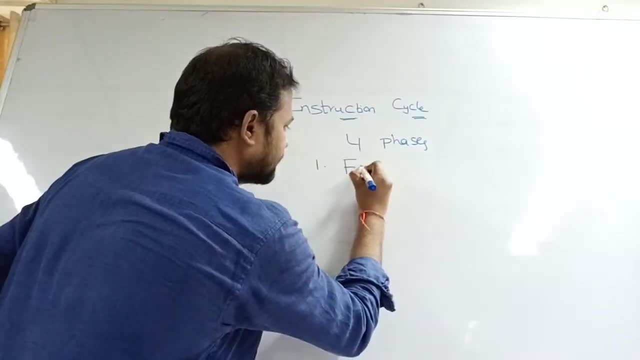 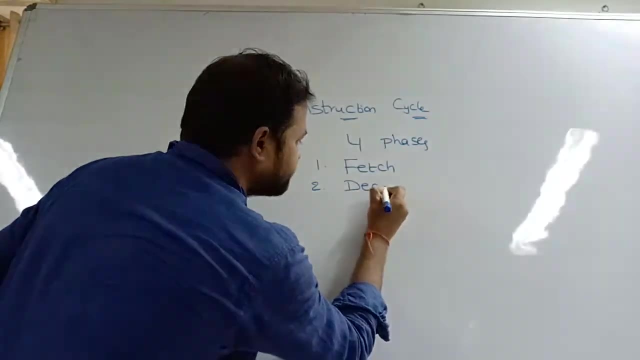 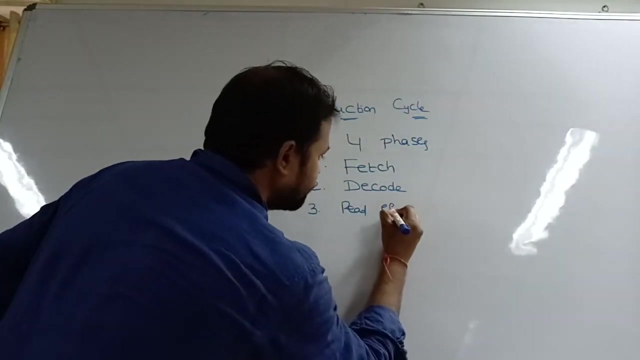 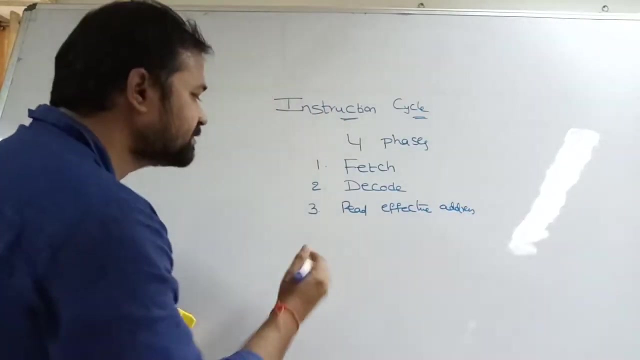 The first page is fetch the instruction from the memory. The second page is decode the instruction. The third page is read effective address If the instruction has indirect address. read effective address If the instruction has indirect address. And the fourth page is execute. 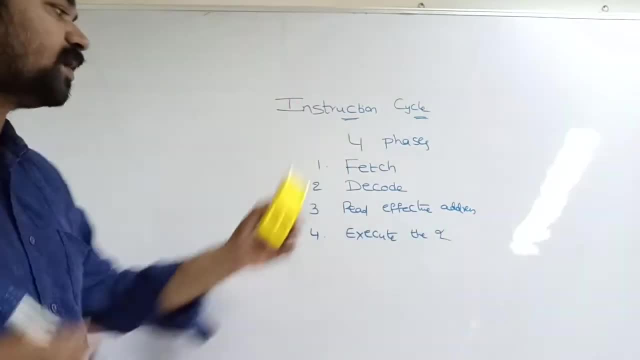 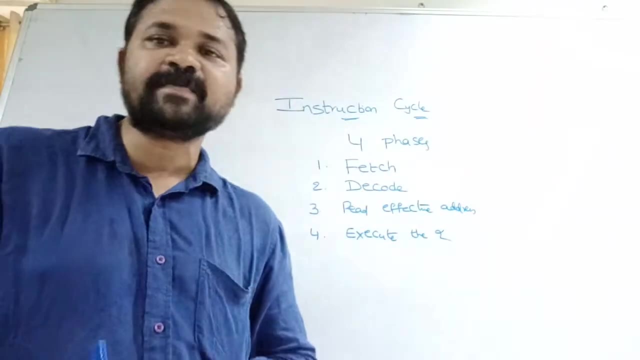 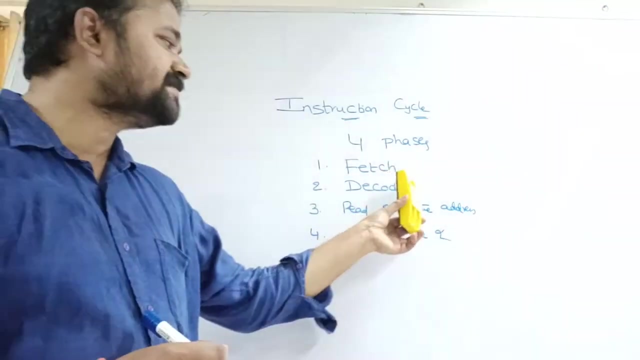 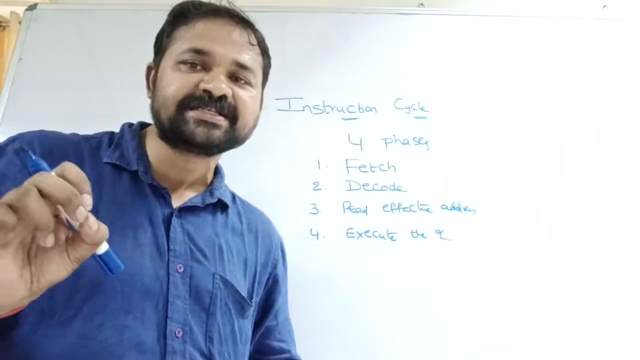 The instruction. So these four are the pages of an instruction cycle. So the first page is fetch, Fetch instruction from the memory. So fetching is nothing but retrieving instruction from the memory. And the second page is decode the instruction. Decoding means determining which operation the corresponding instruction will perform. And the third page is read: effective address. 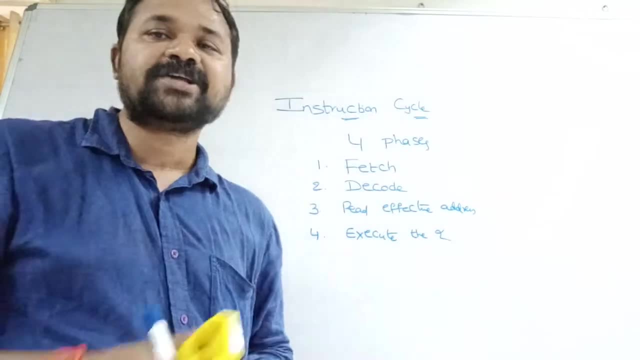 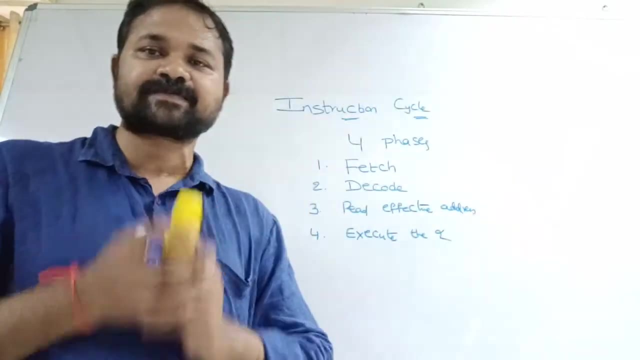 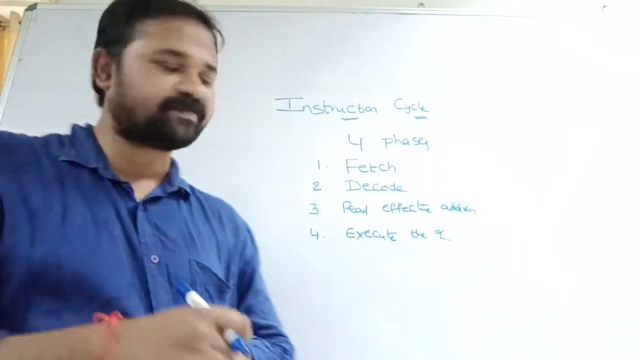 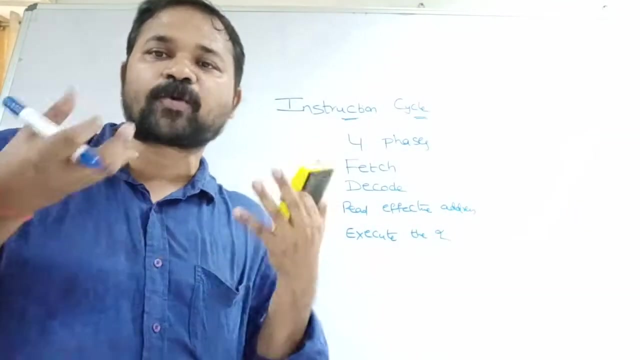 If the instruction has an indirect bit. Generally every instruction contains indirect bit. If indirect bit is one, then it is called as indirect address. So if the instruction is an indirect instruction, then we have to determine the effective address. So that is the third page And the fourth page is execute the instruction. So first let us assume that our program contains 10 instructions. 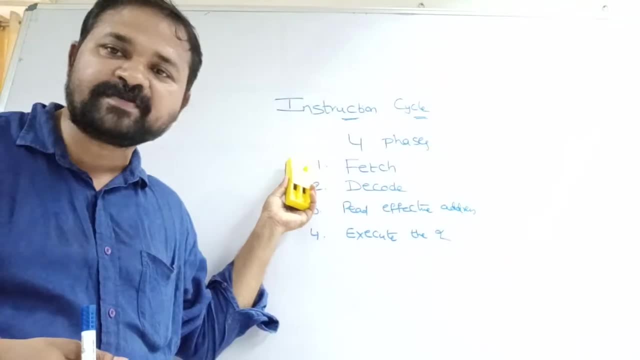 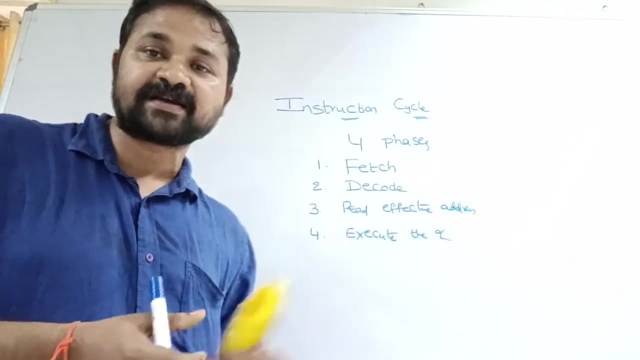 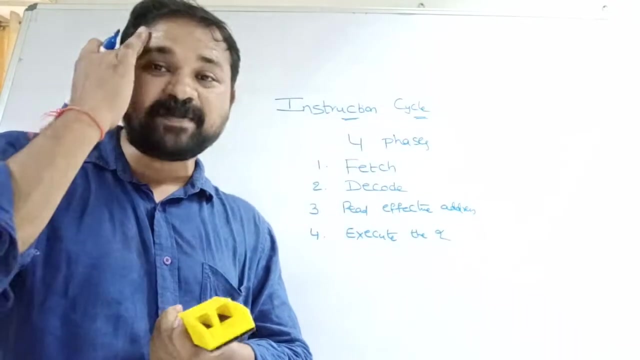 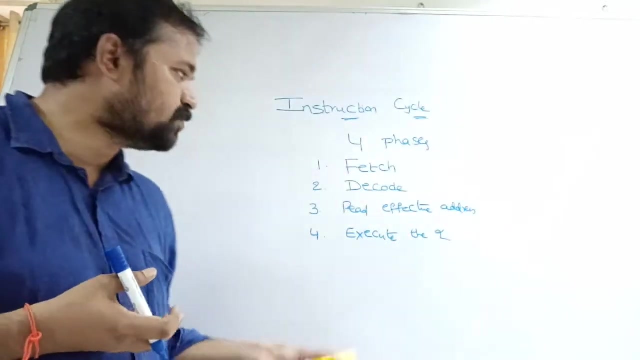 So first, the first instruction will be fetched from the memory. The first instruction will be decoded. Next, for the first instruction, this effective address will be determined. Next, the first instruction will be executed. So now the first instruction execution is over. Now CPU starts executing the second instruction. So now the second instruction instruction cycle will be executed by using these four pages. 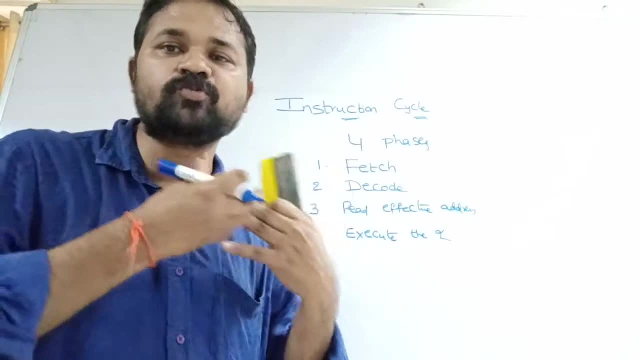 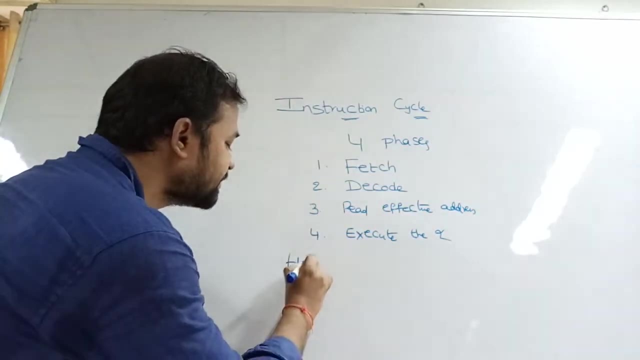 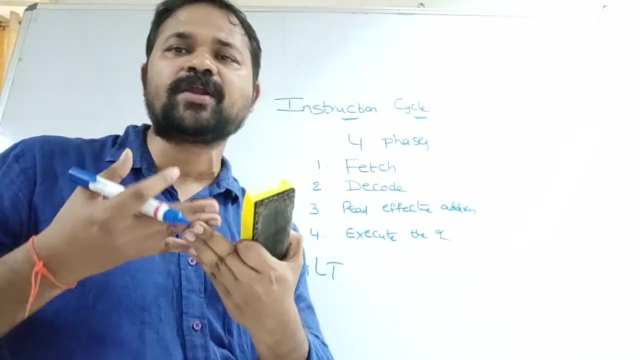 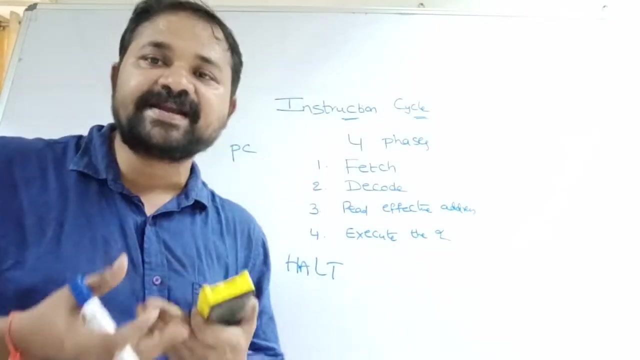 So likewise, all the instructions in the program are to be executed. The last instruction of any program is halt. So whenever this halt instruction is executed, then the program execution will be over. Now let us see what is a program counter. So we have a register called program counter. Program counter always contains address of next instruction to be executed. 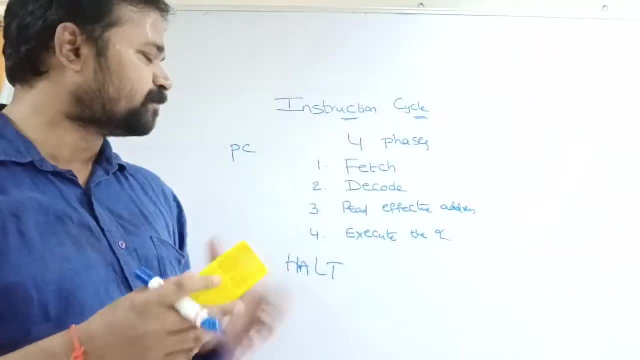 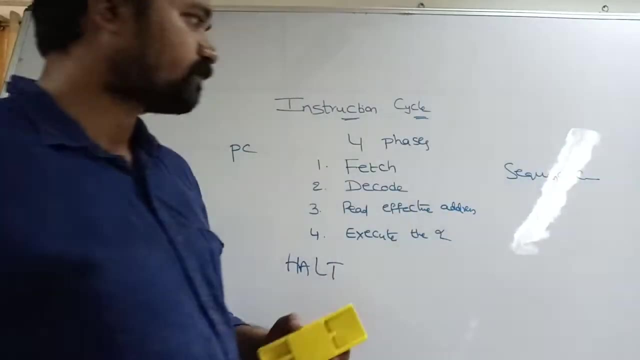 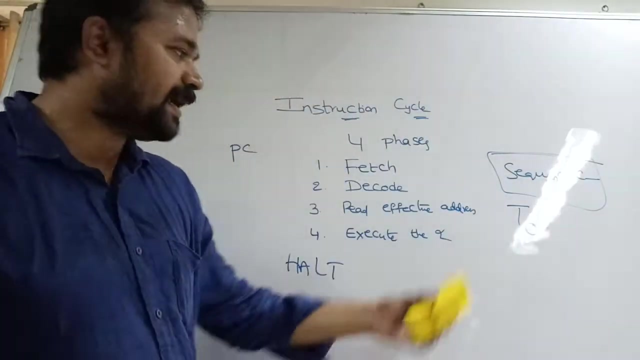 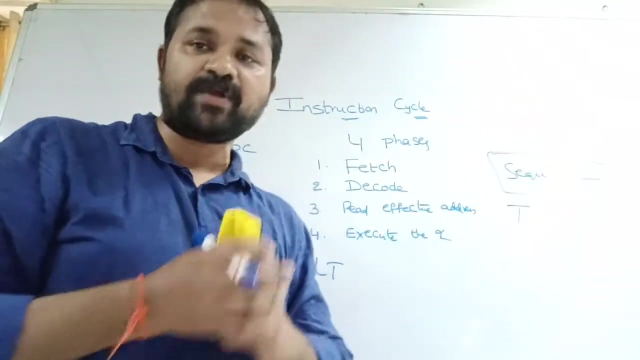 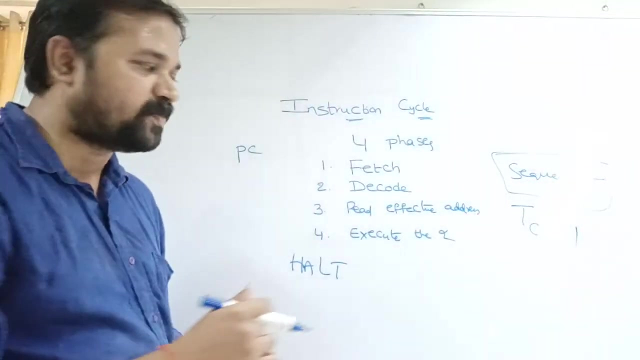 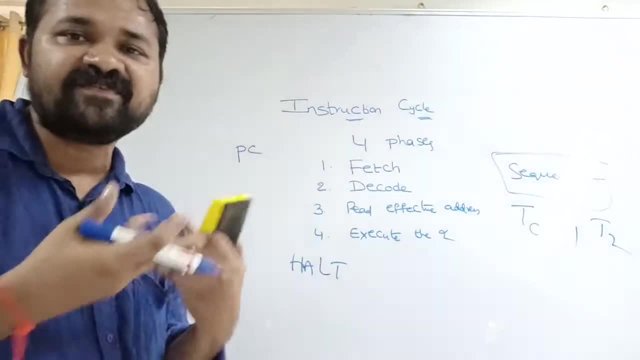 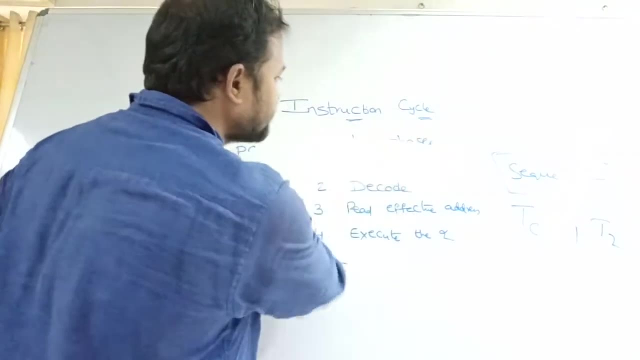 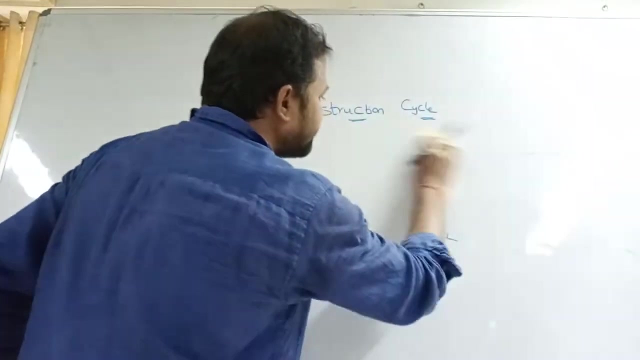 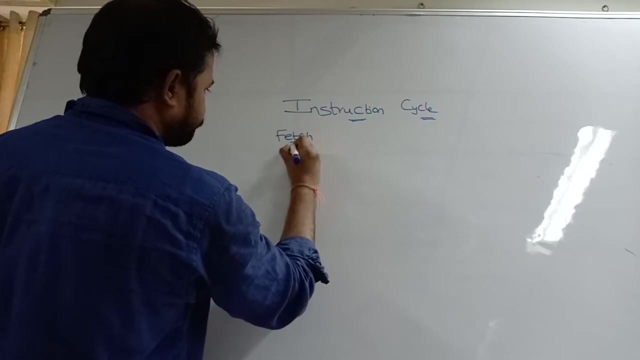 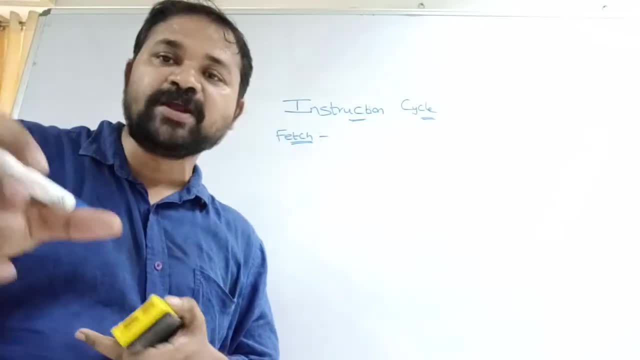 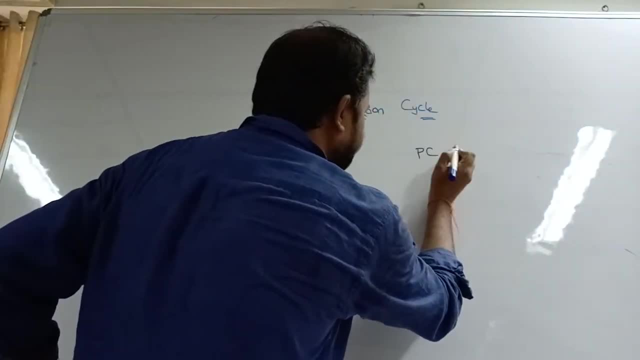 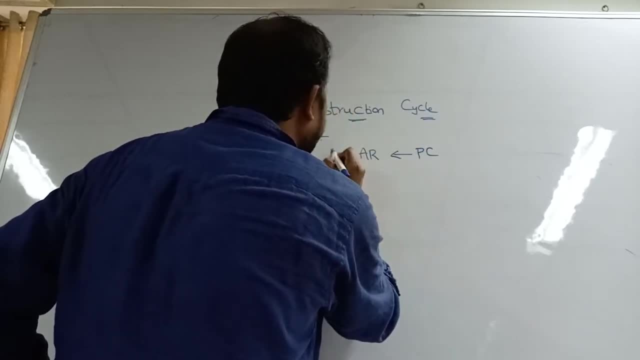 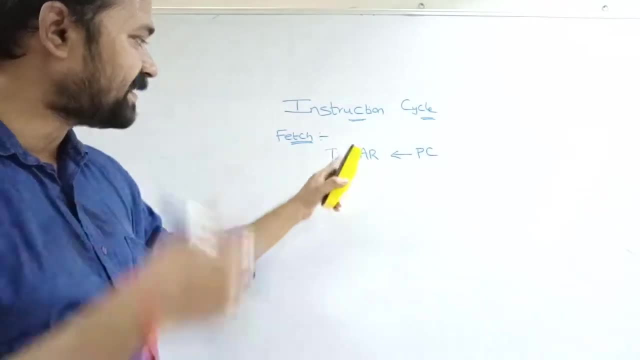 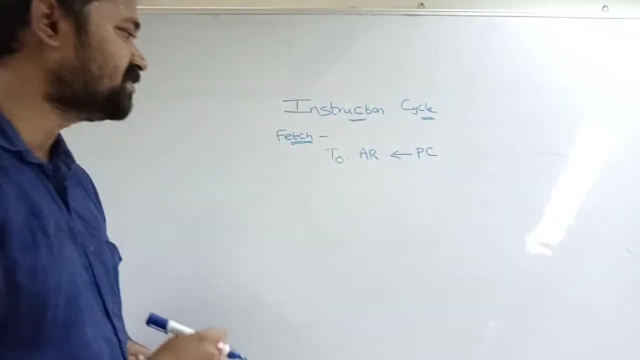 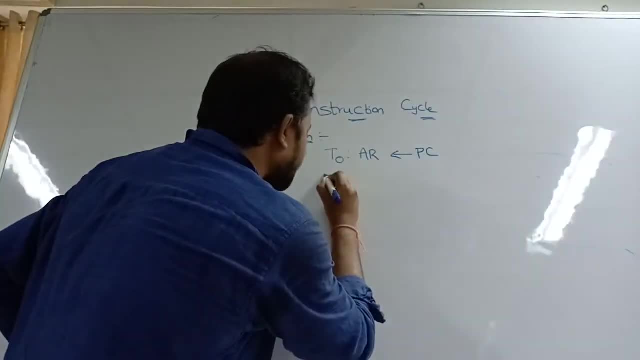 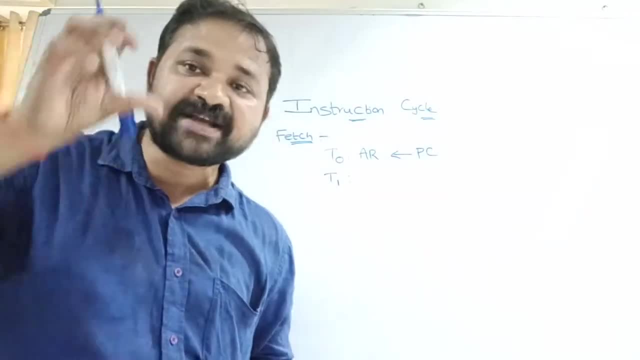 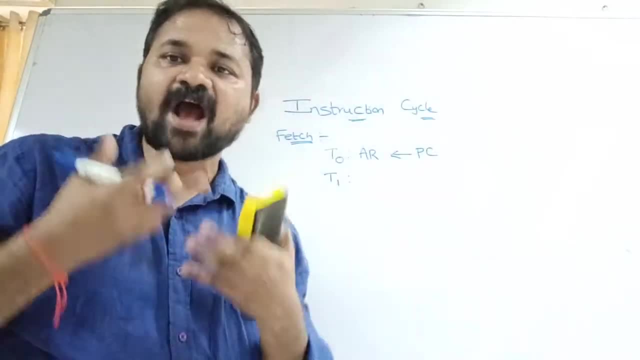 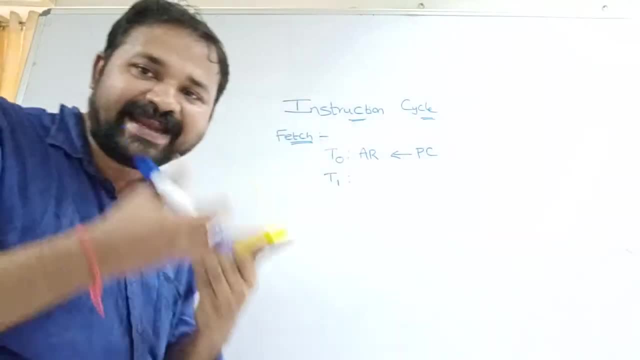 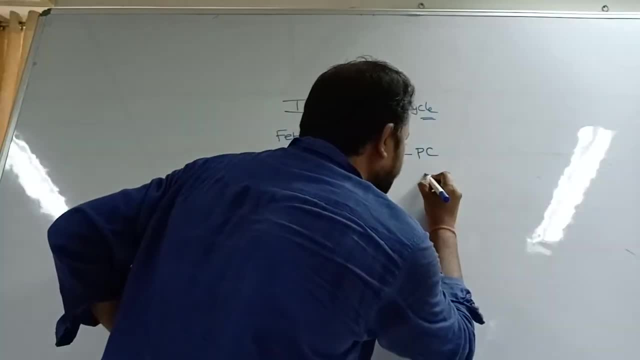 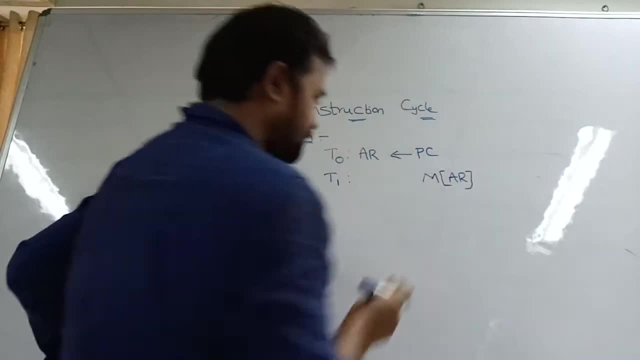 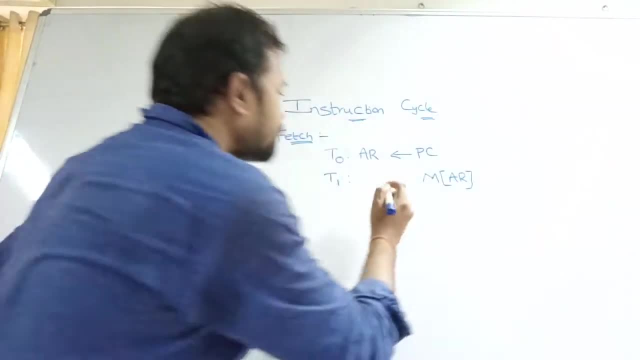 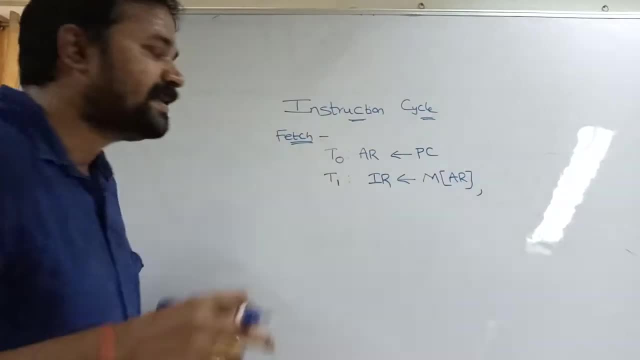 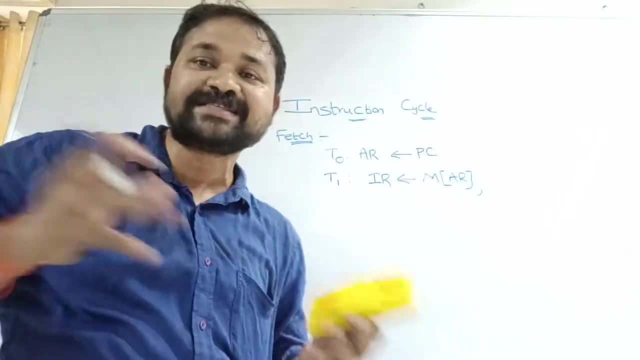 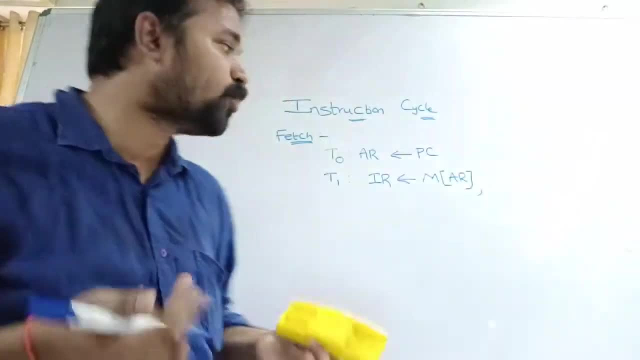 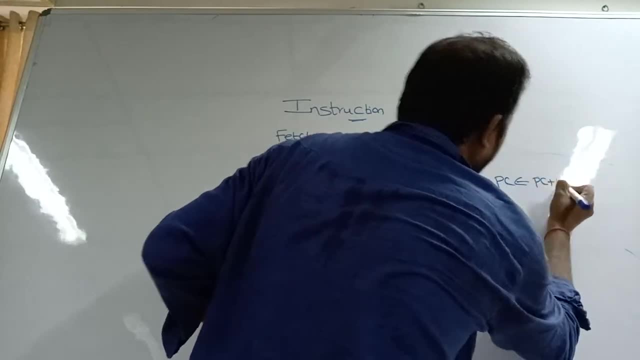 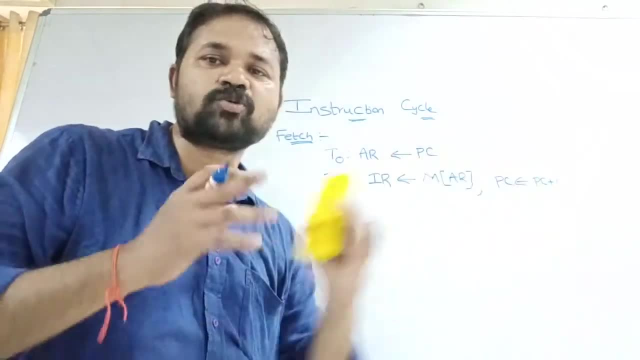 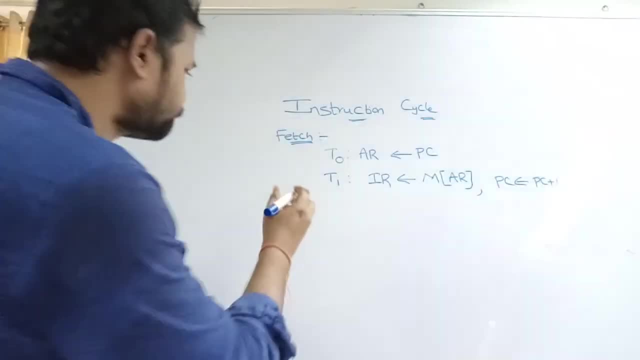 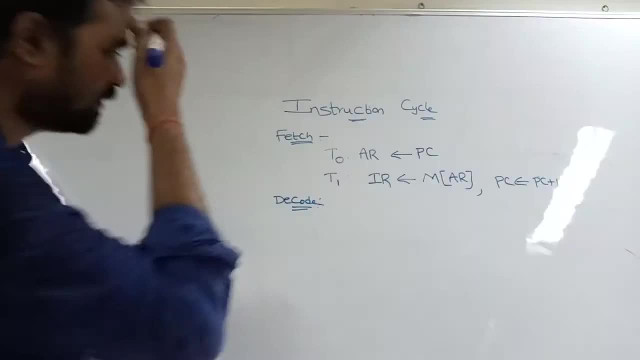 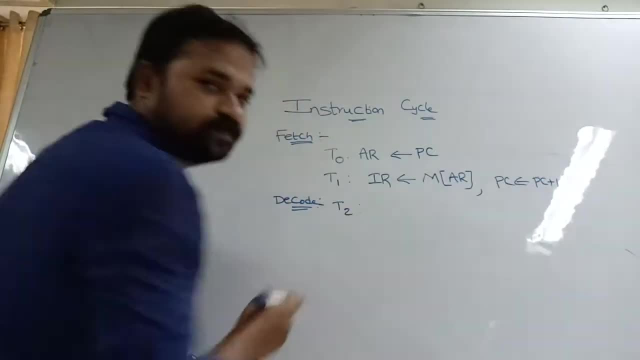 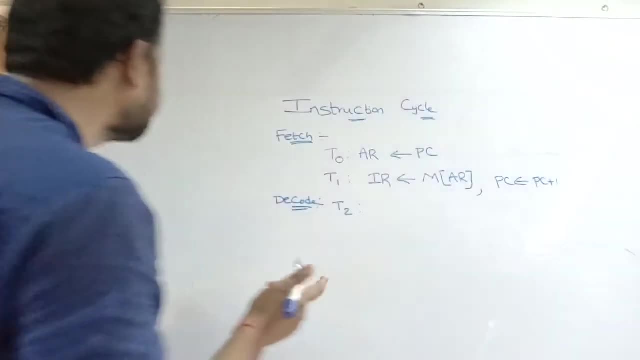 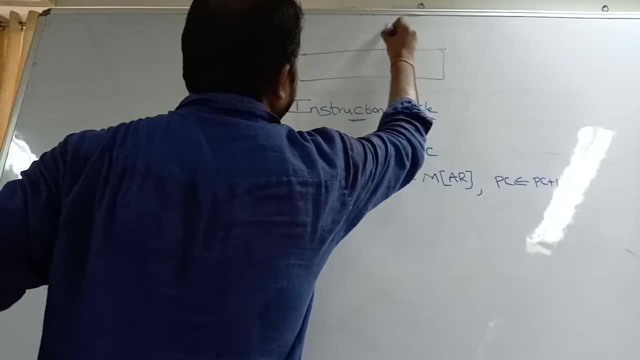 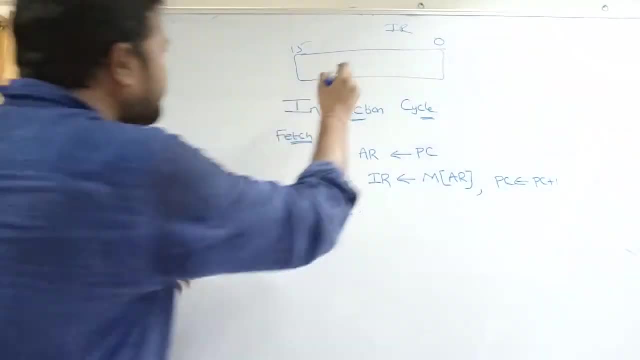 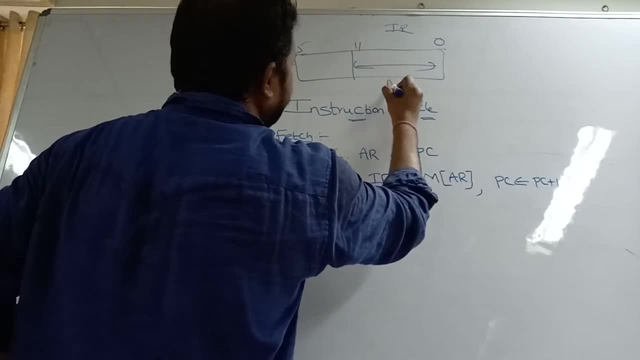 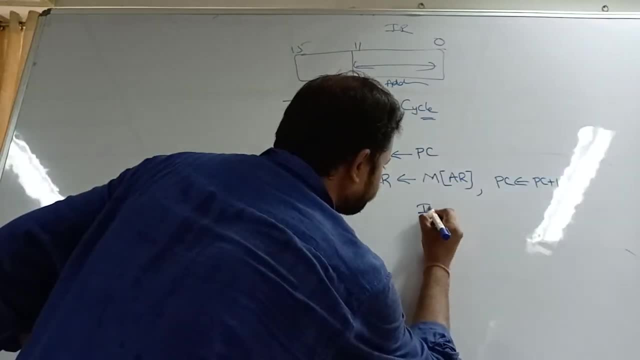 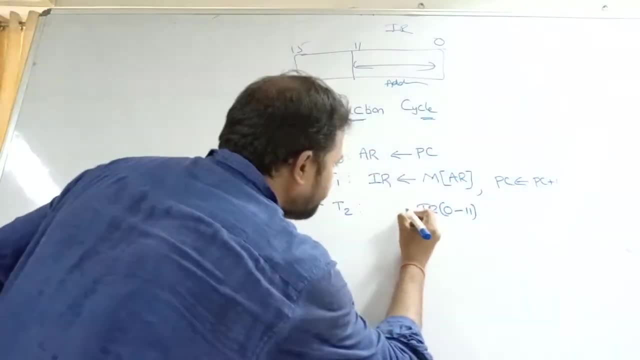 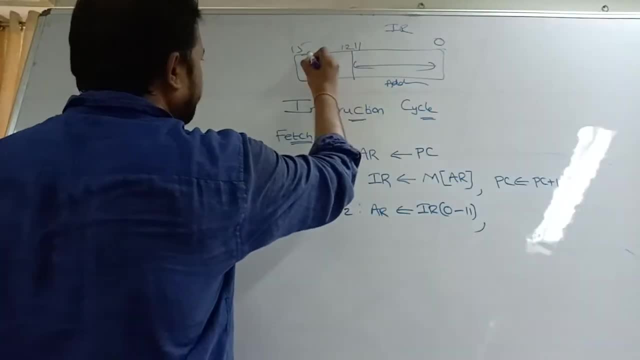 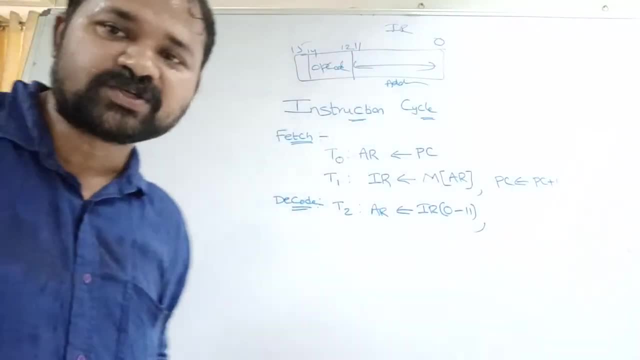 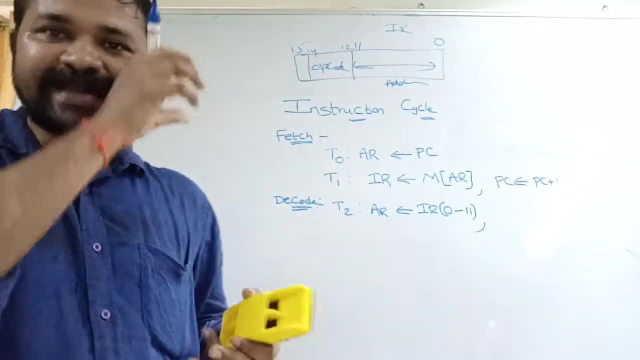 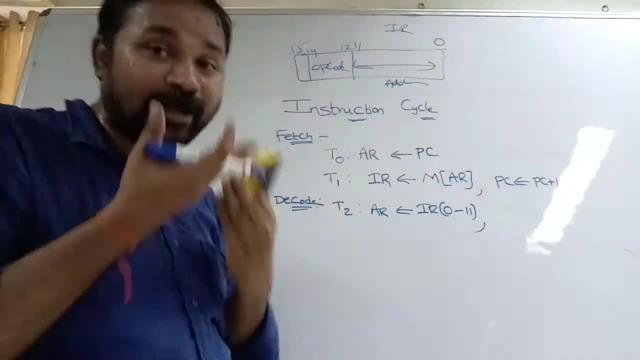 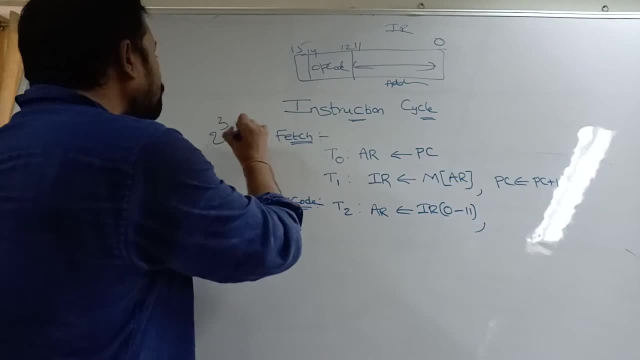 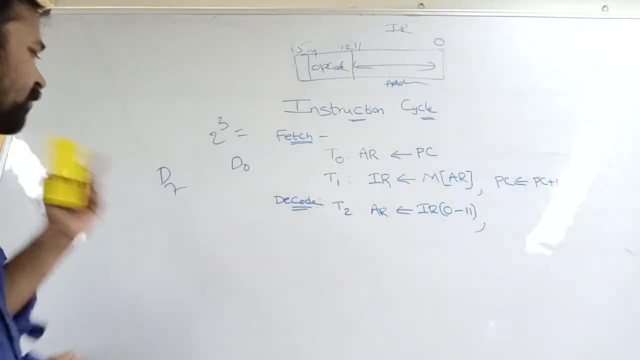 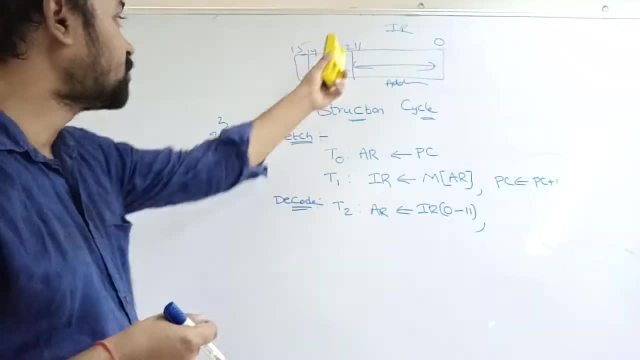 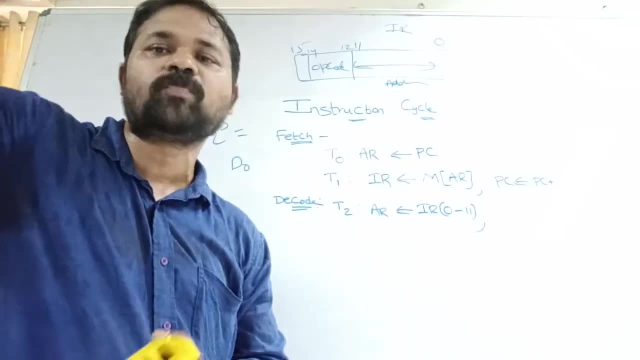 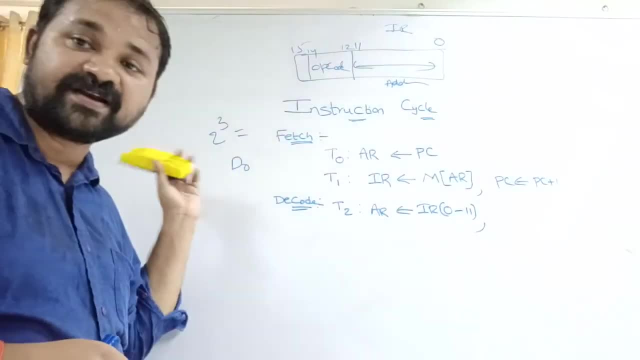 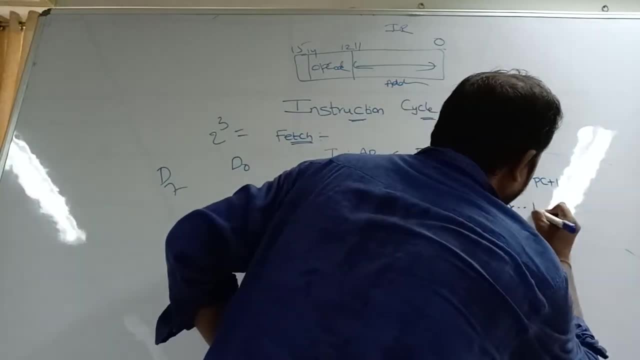 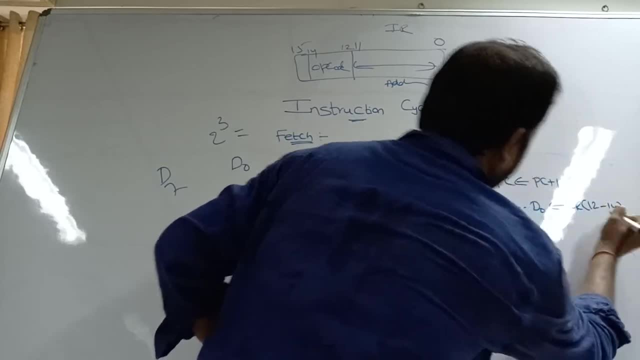 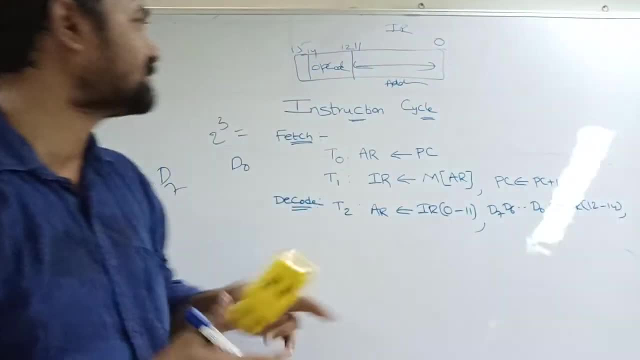 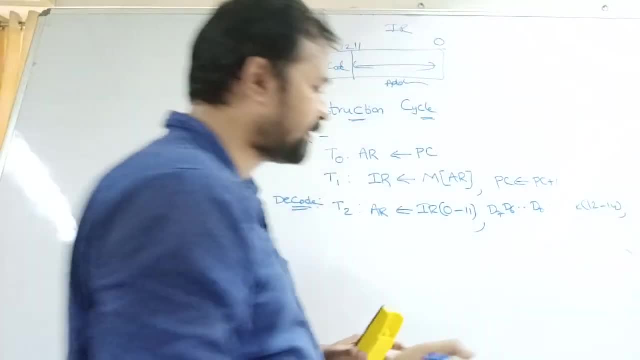 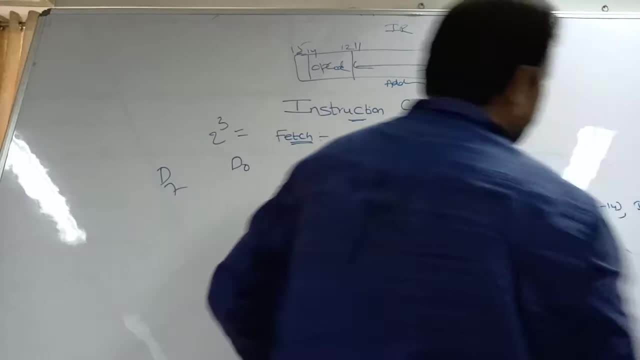 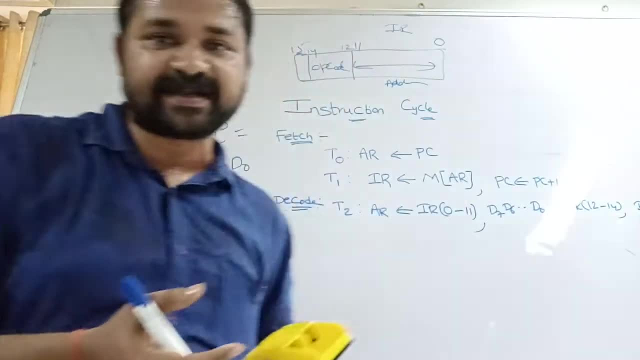 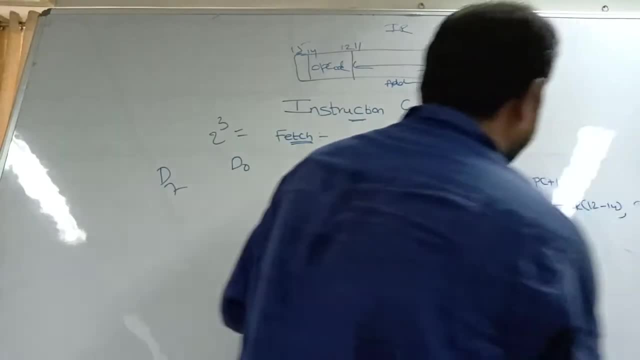 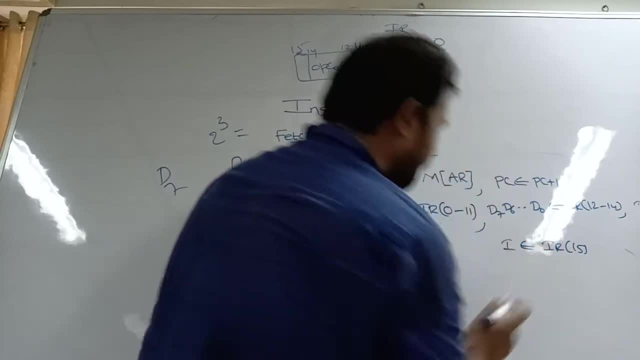 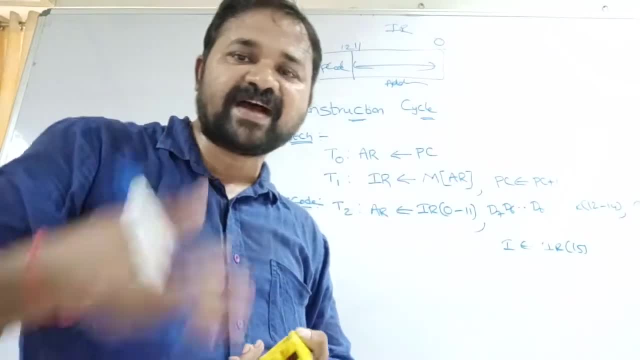 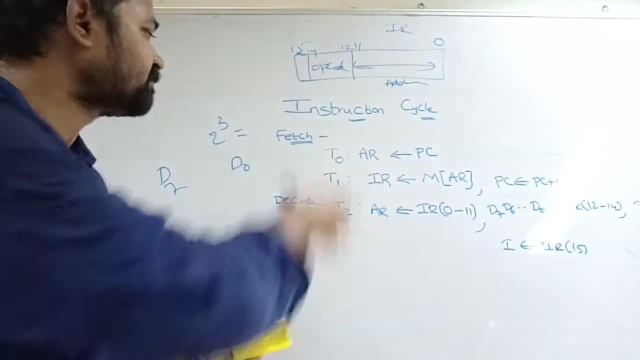 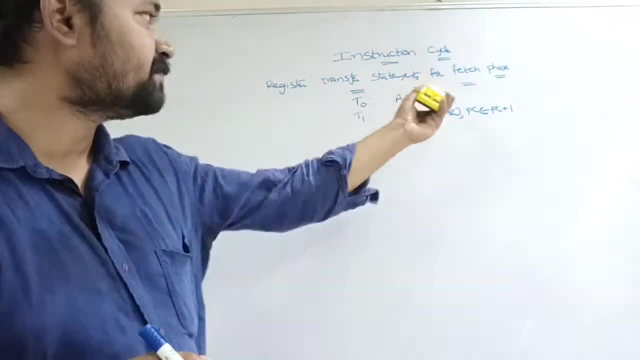 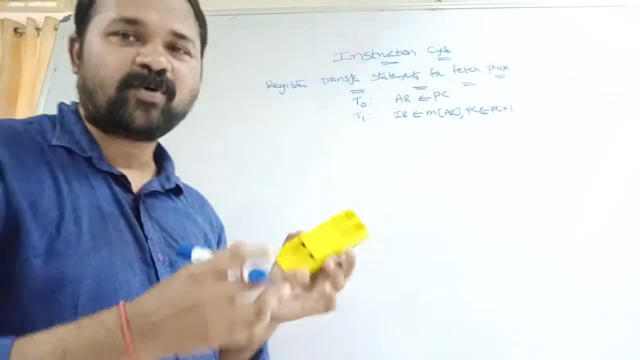 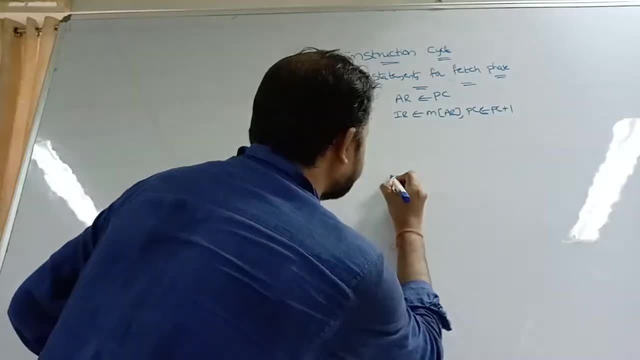 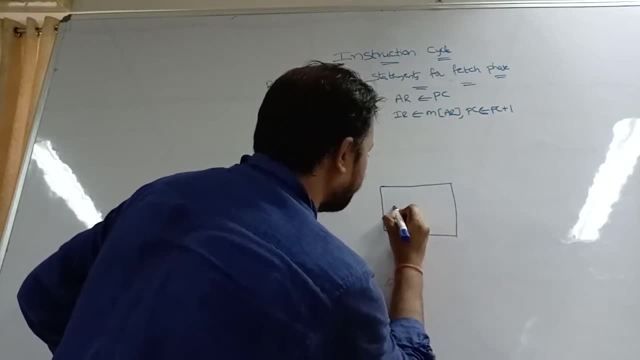 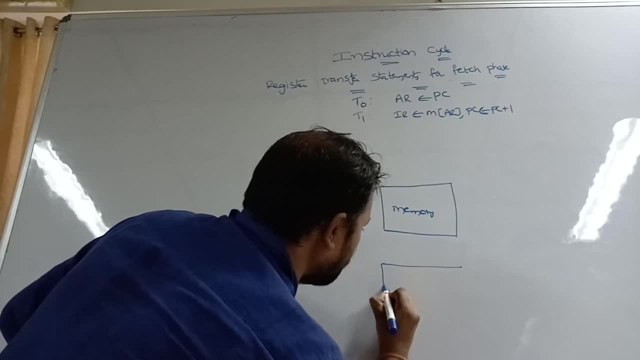 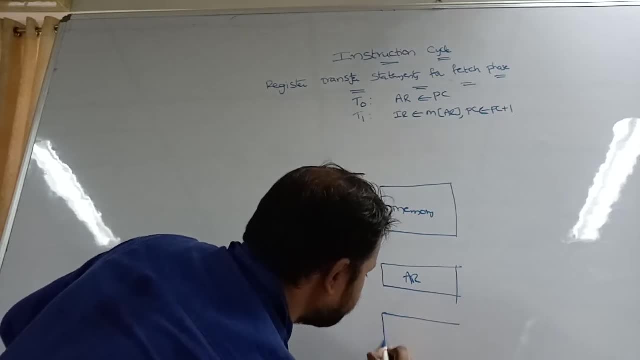 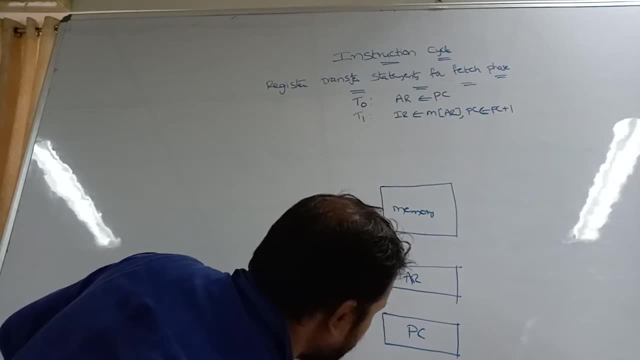 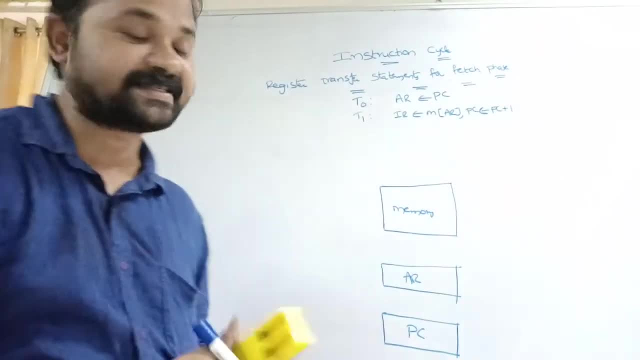 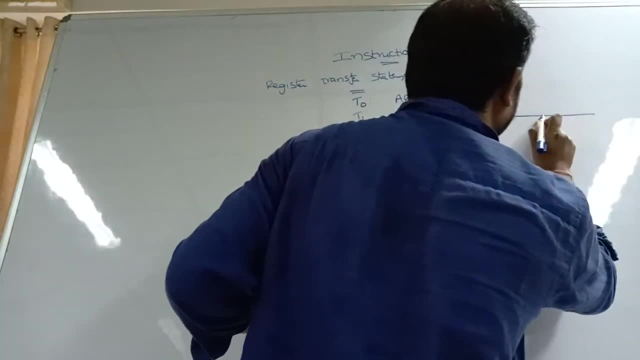 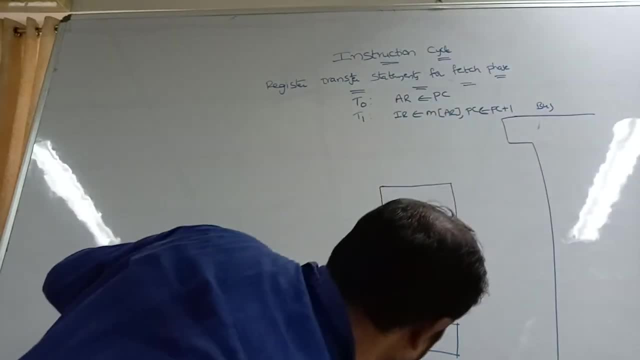 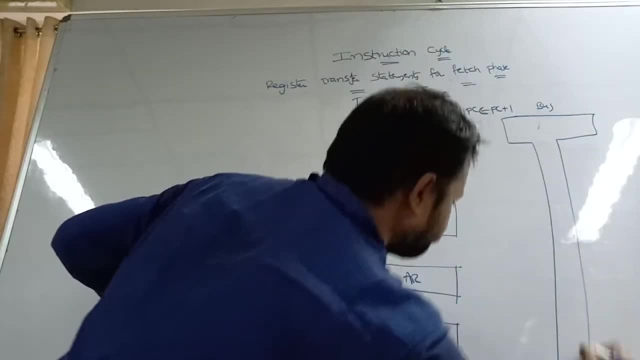 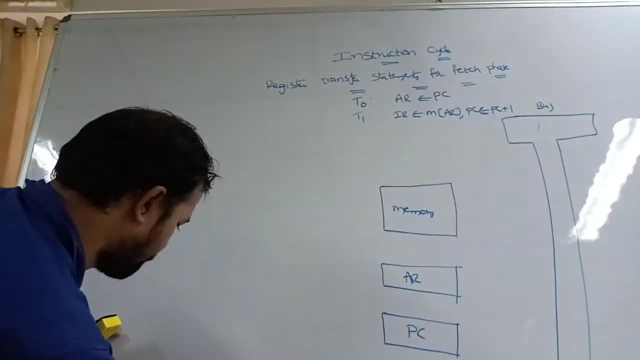 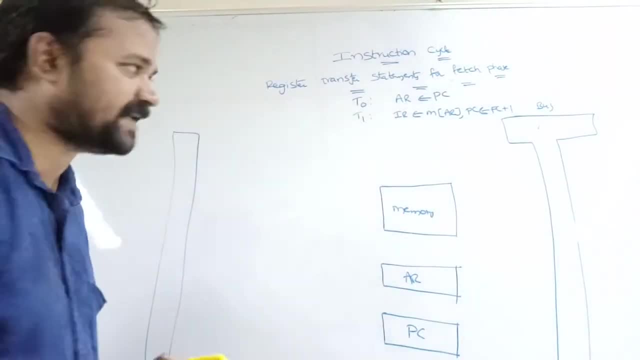 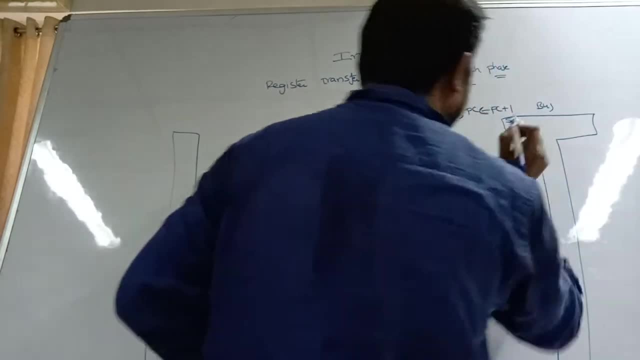 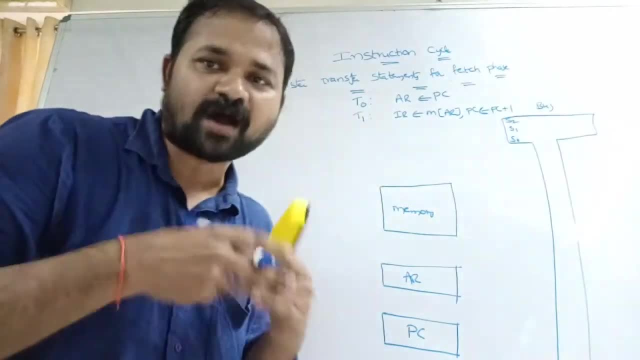 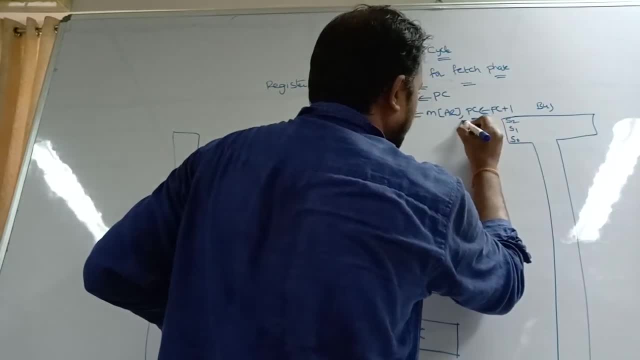 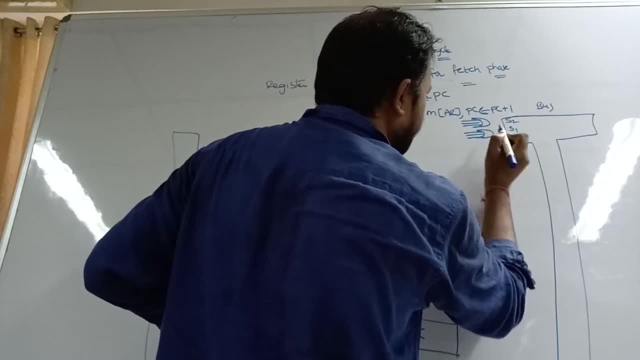 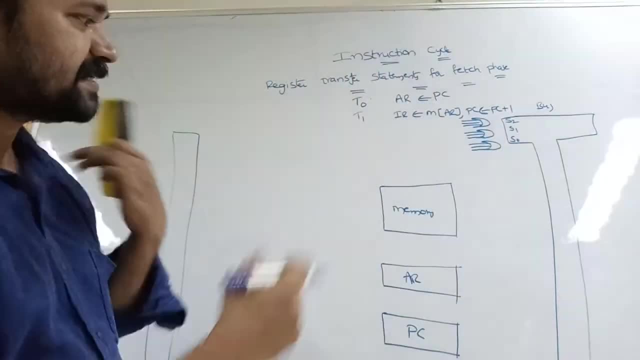 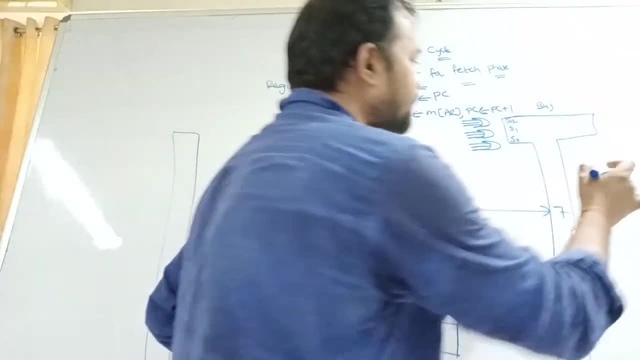 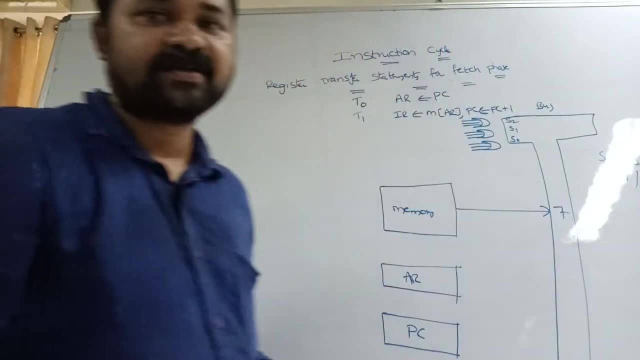 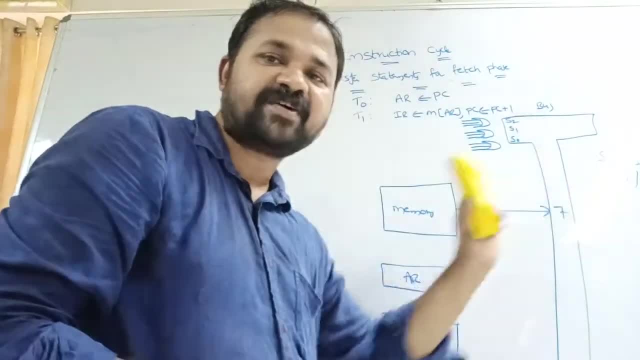 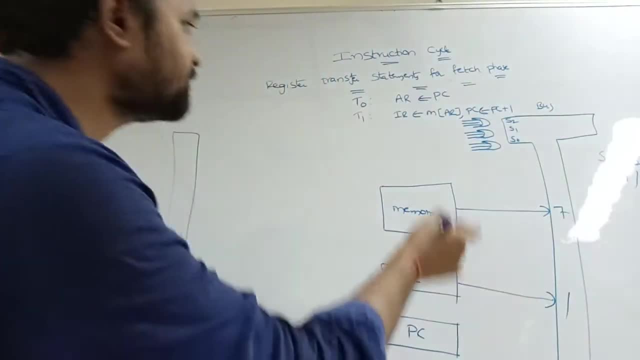 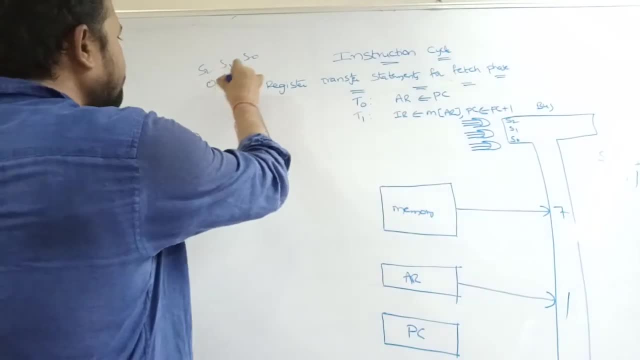 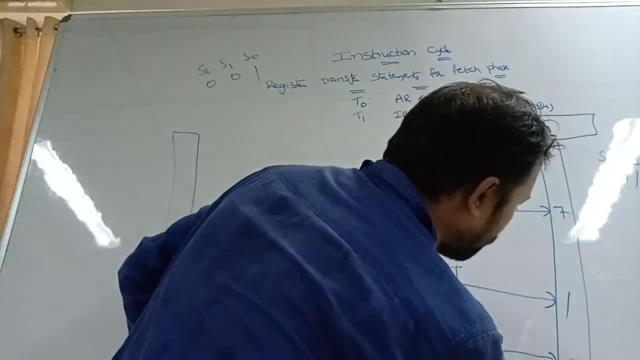 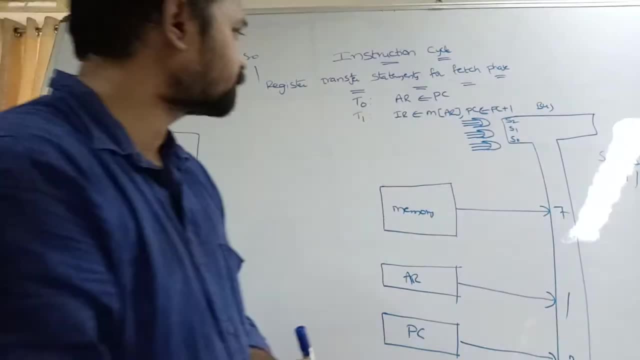 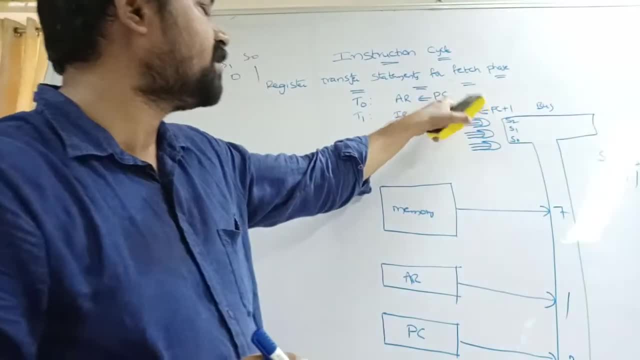 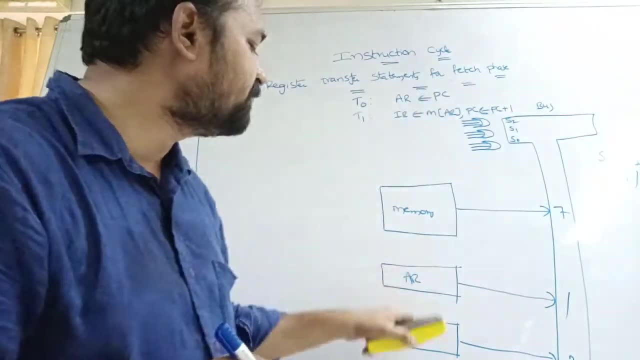 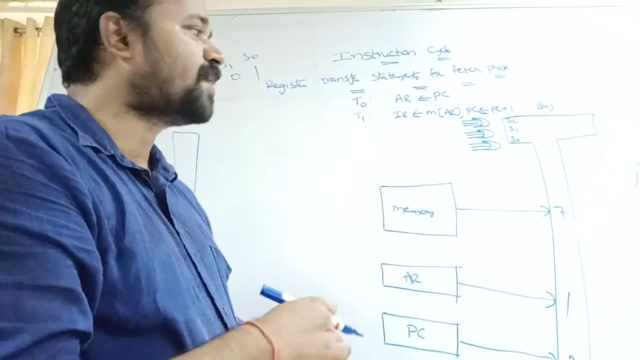 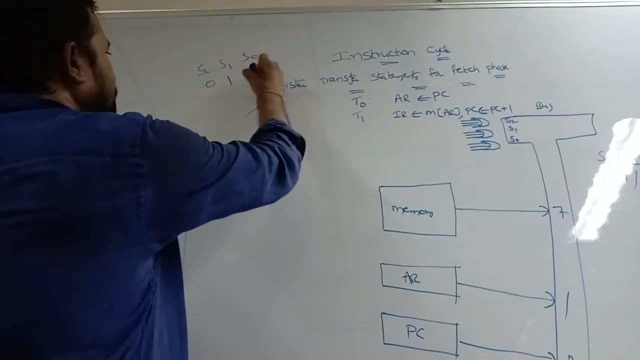 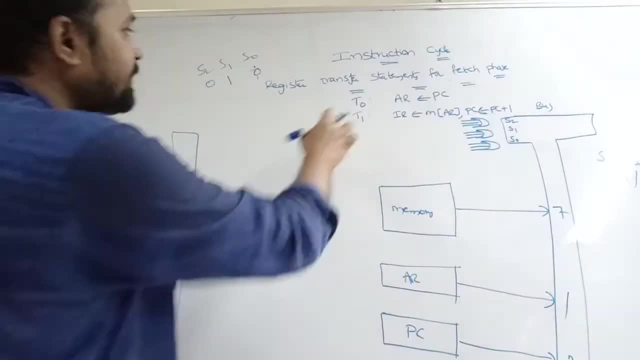 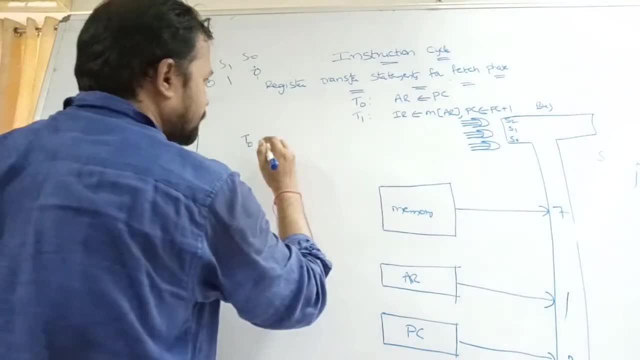 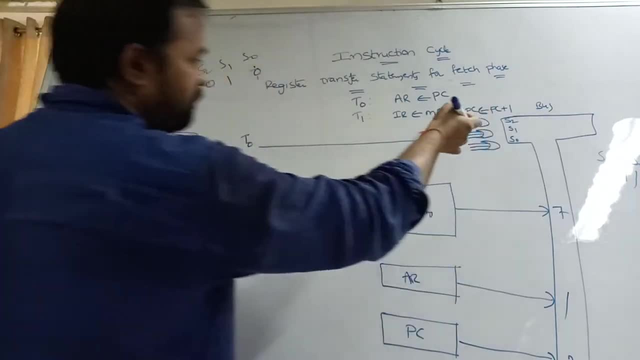 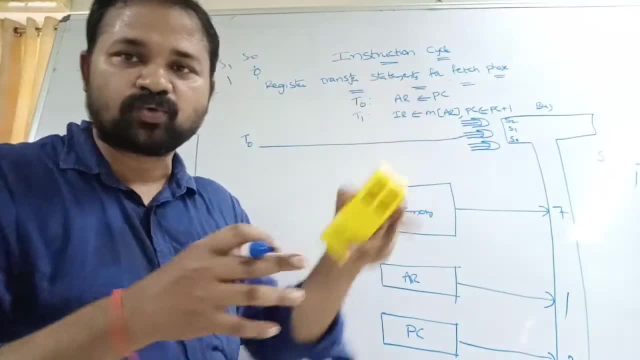 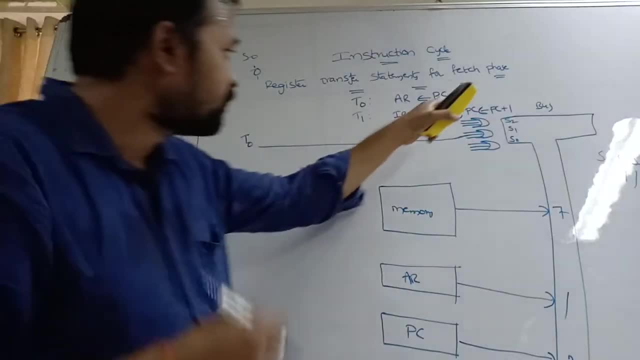 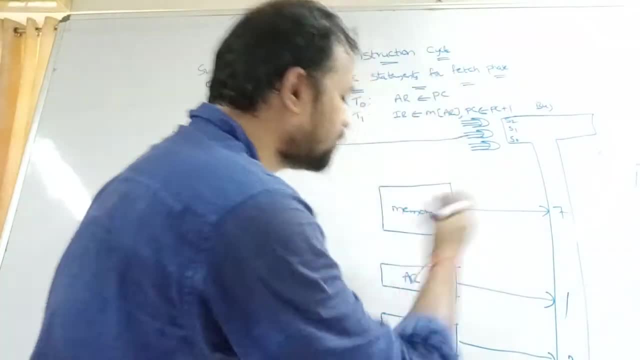 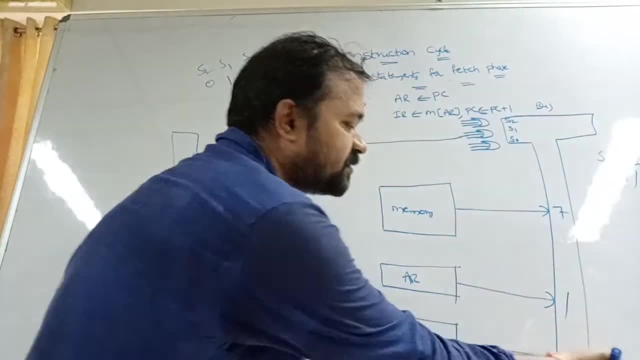 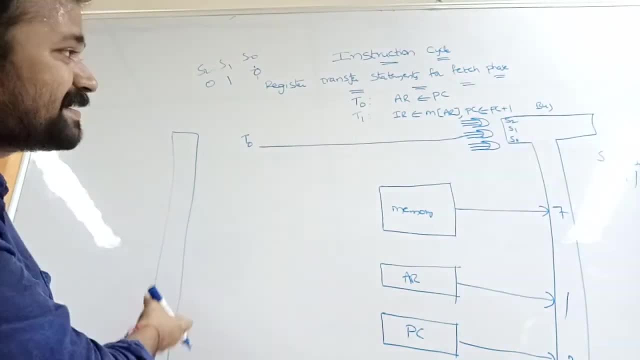 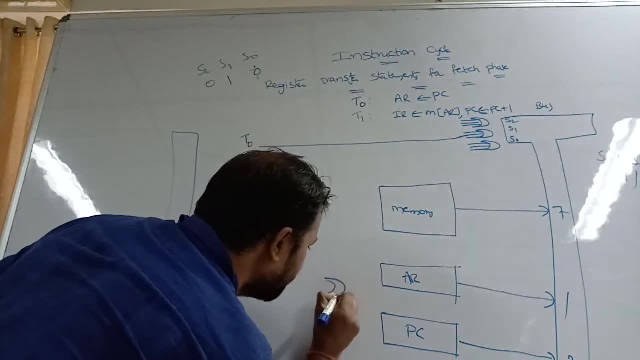 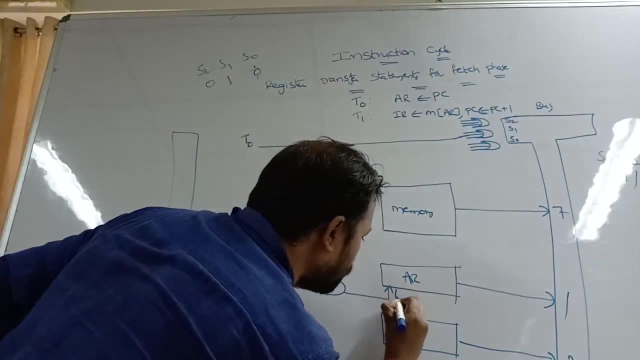 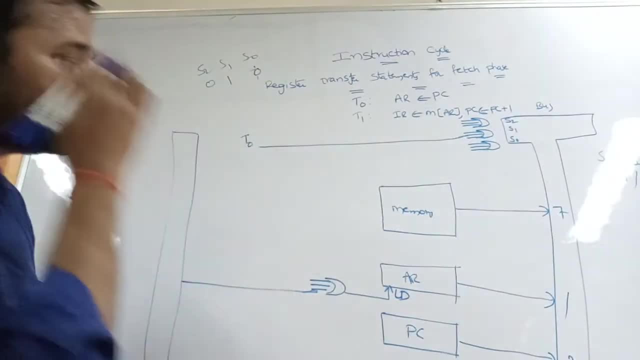 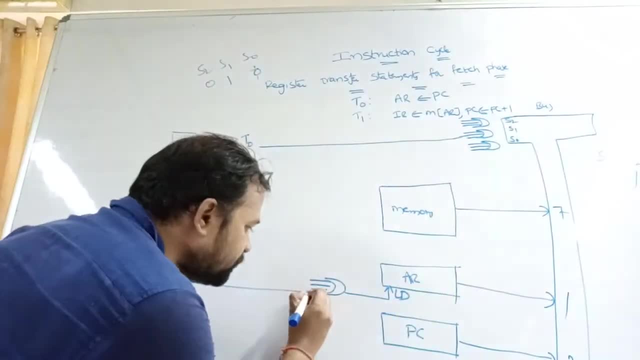 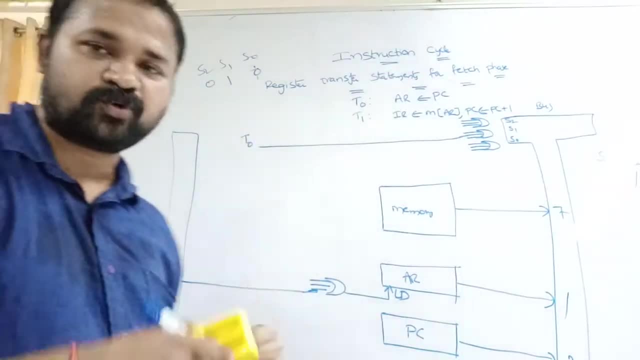 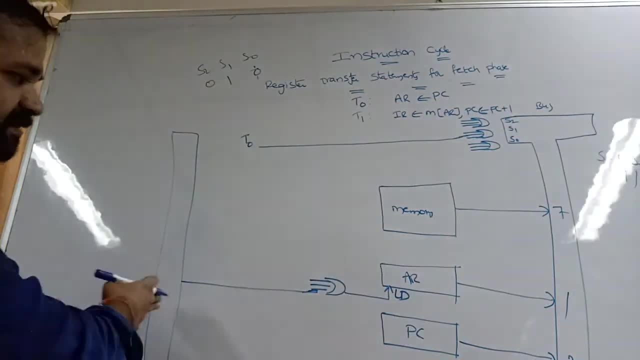 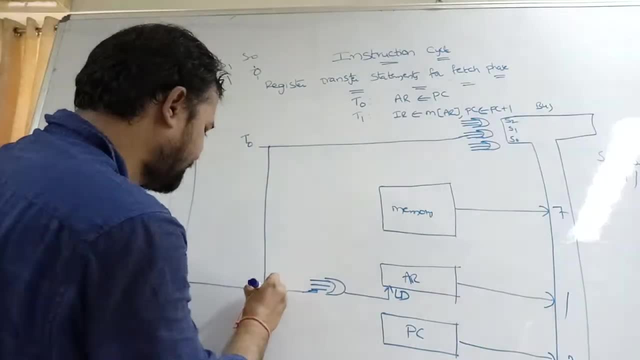 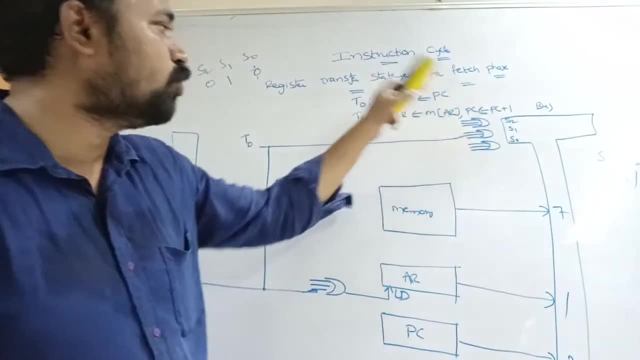 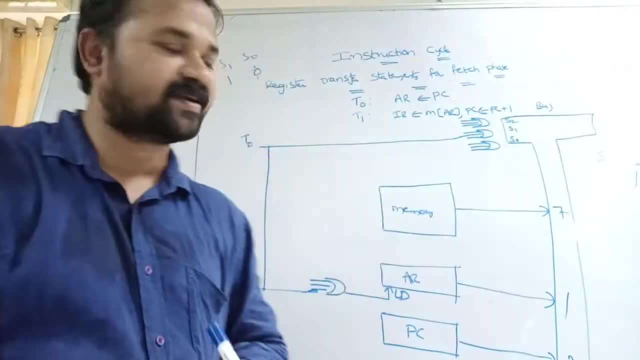 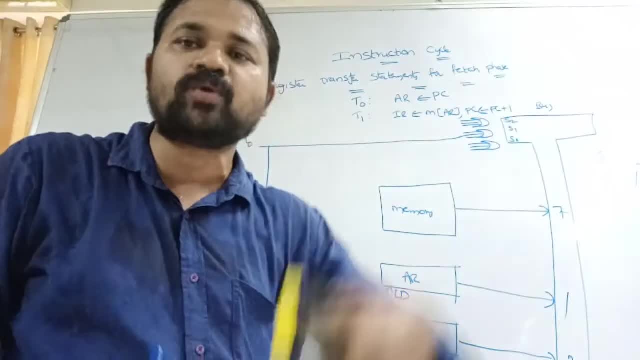 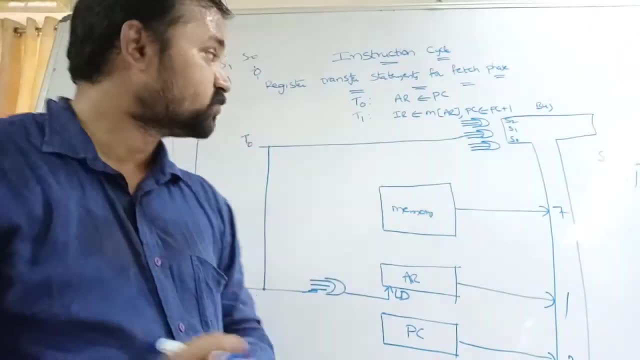 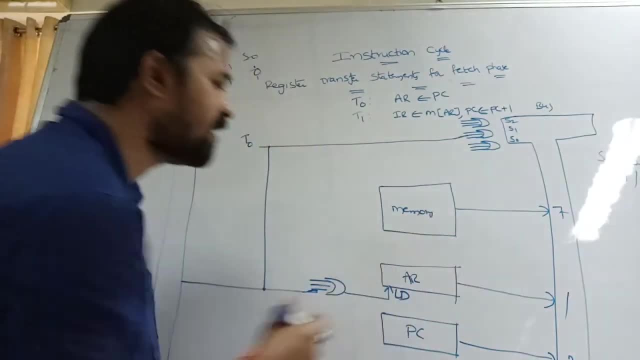 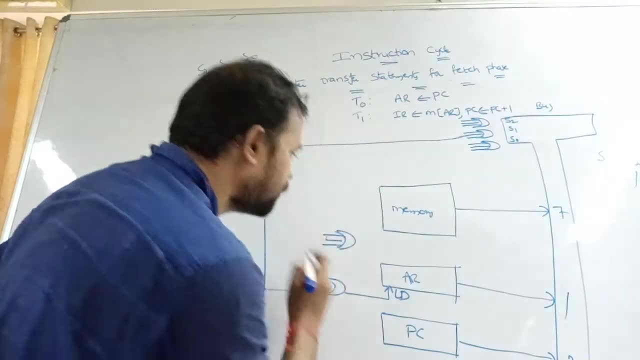 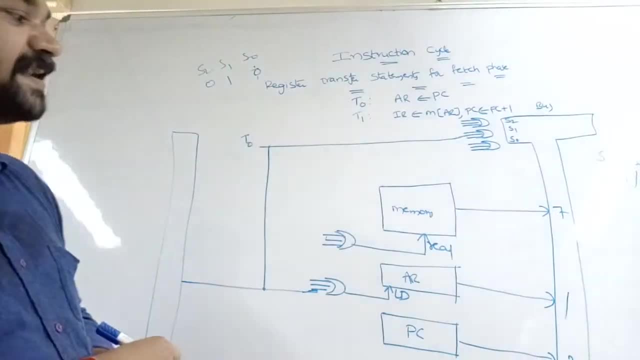 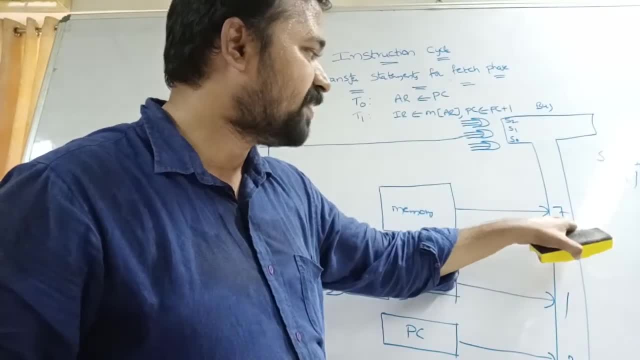 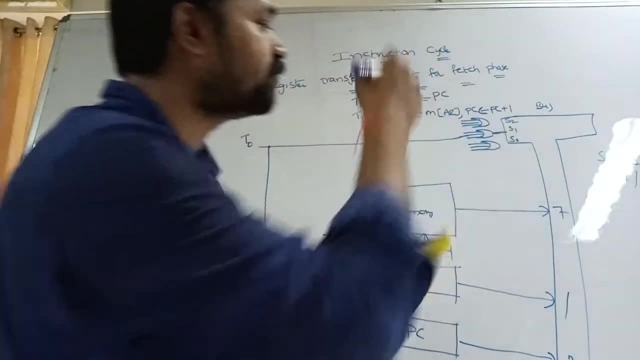 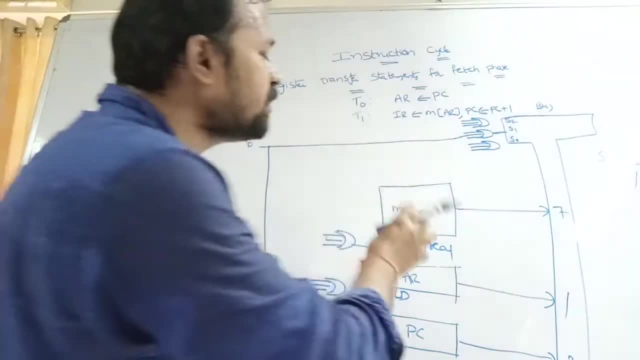 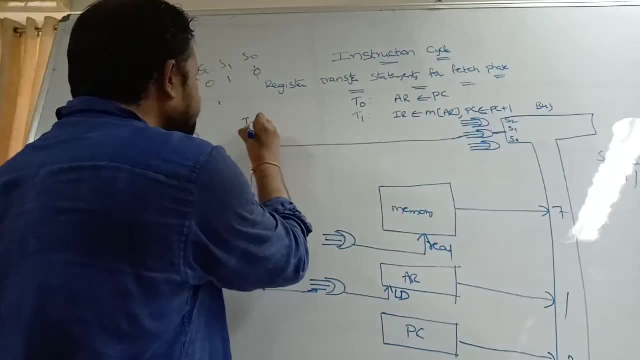 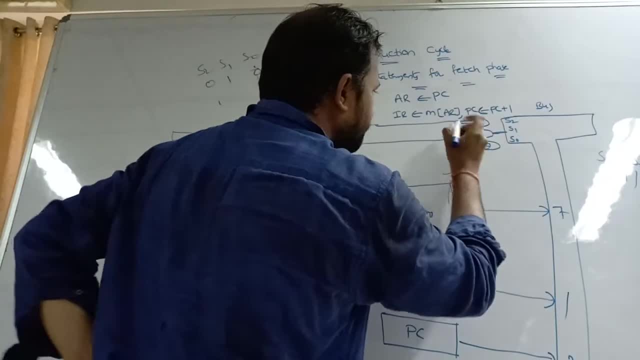 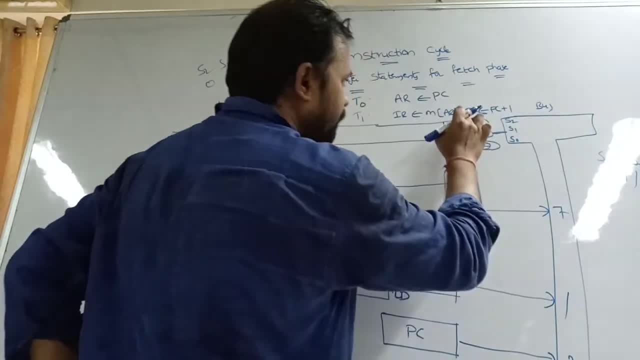 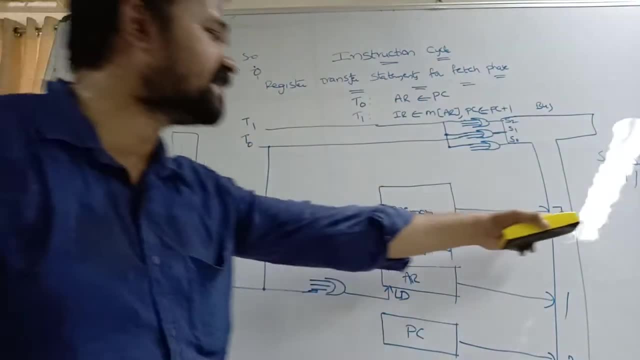 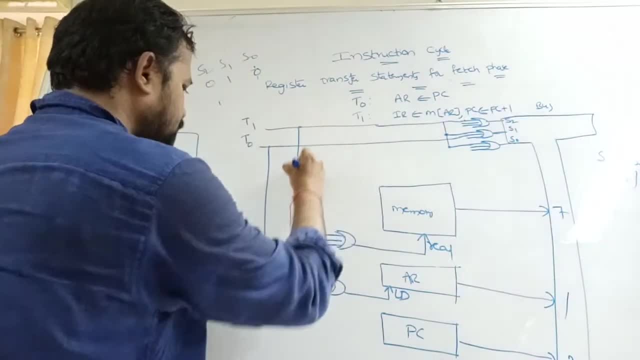 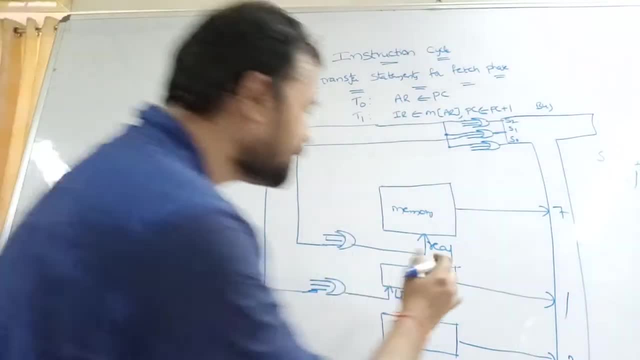 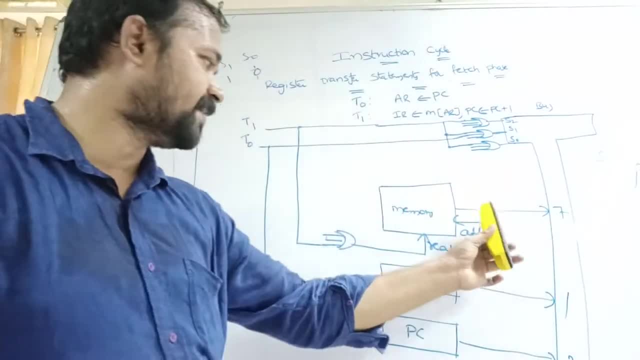 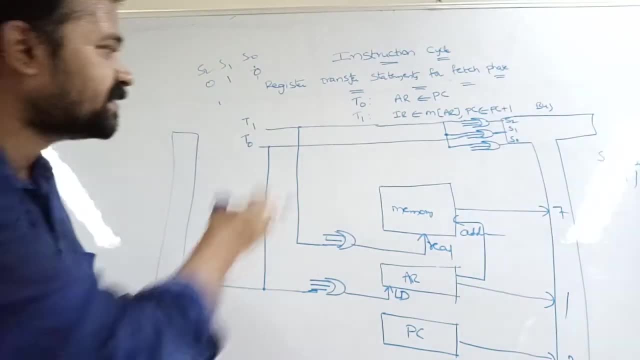 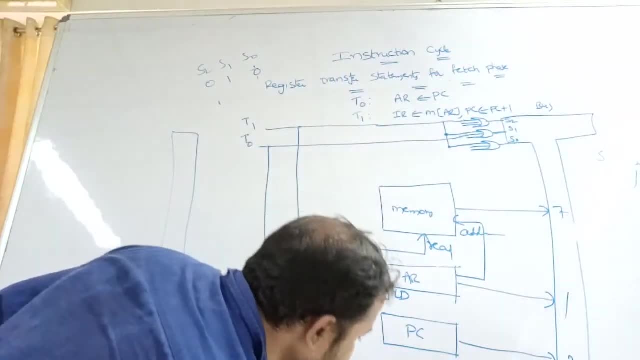 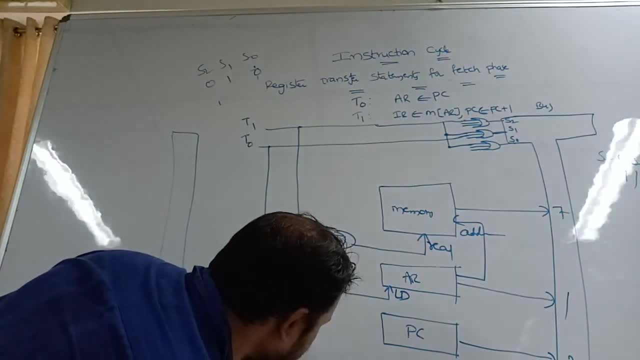 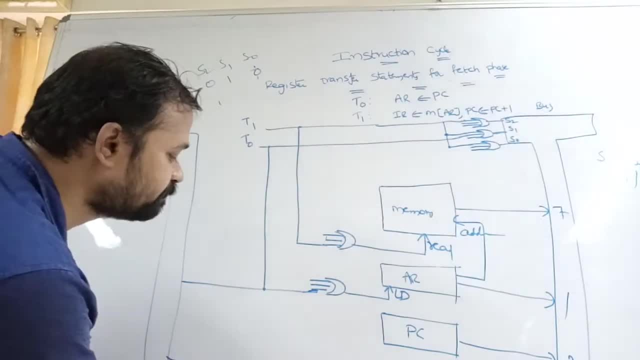 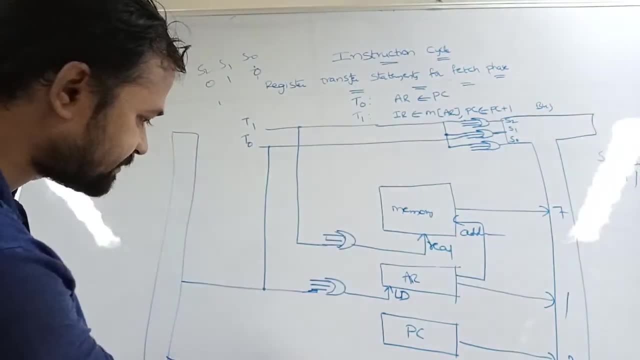 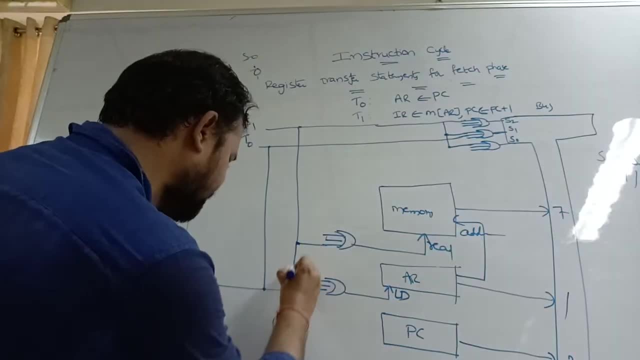 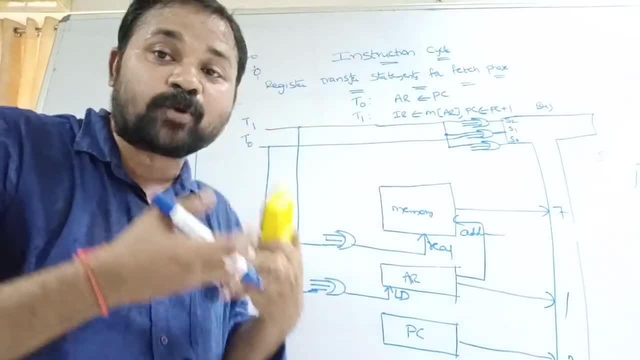 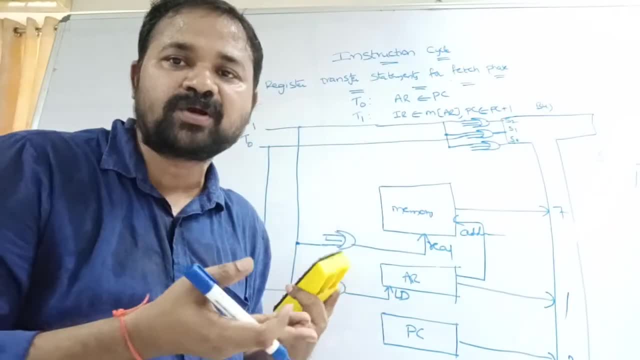 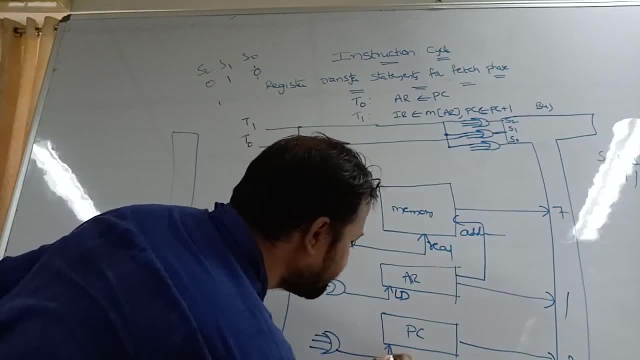 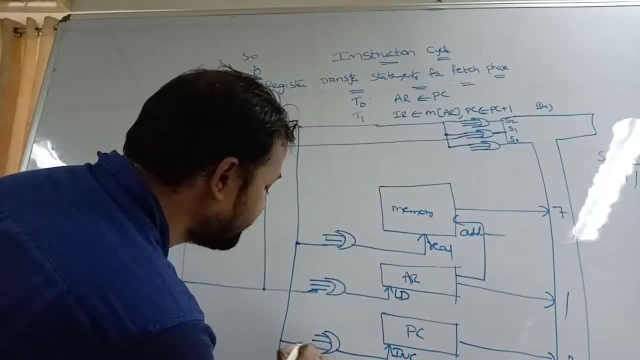 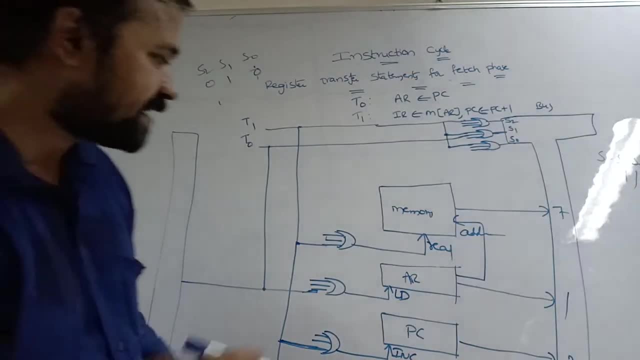 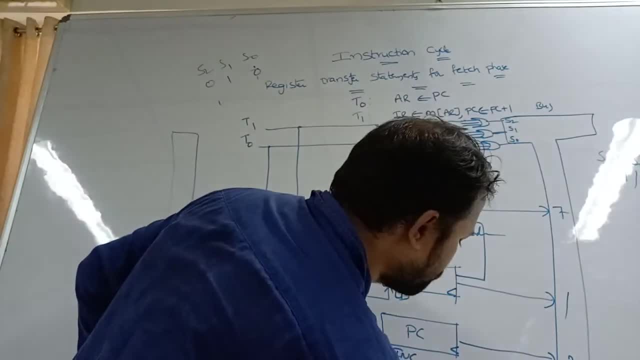 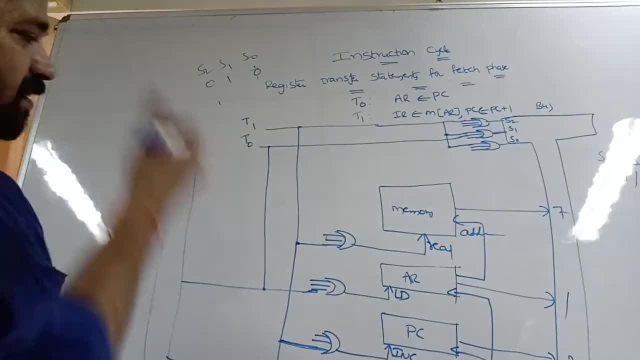 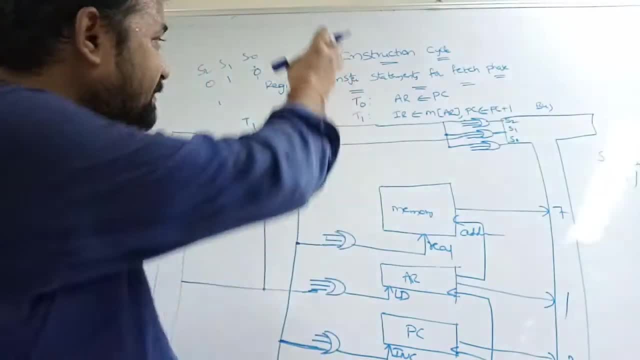 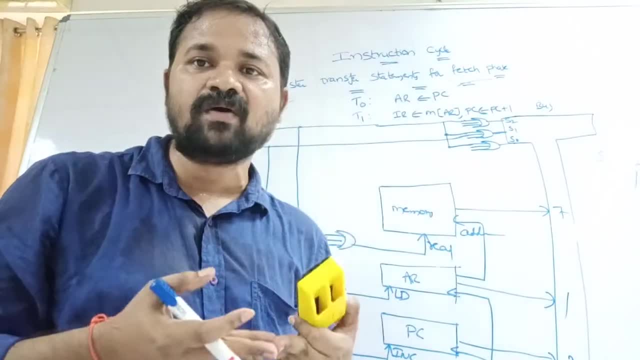 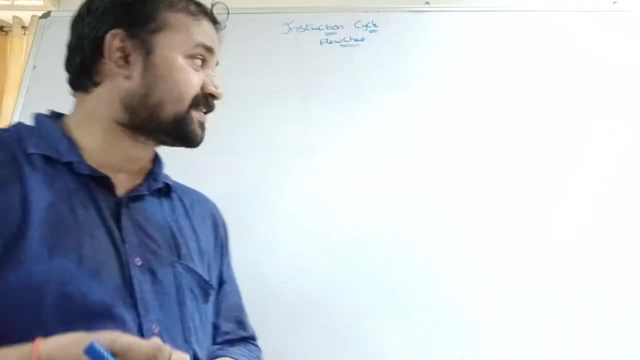 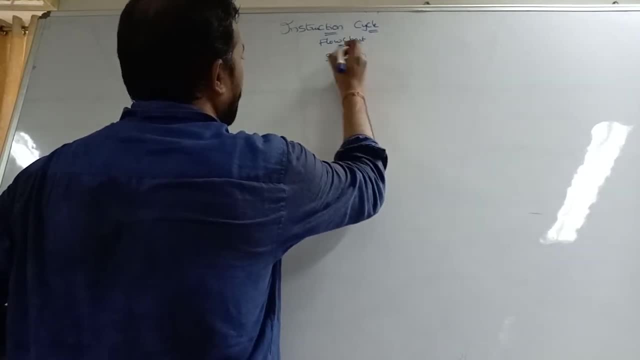 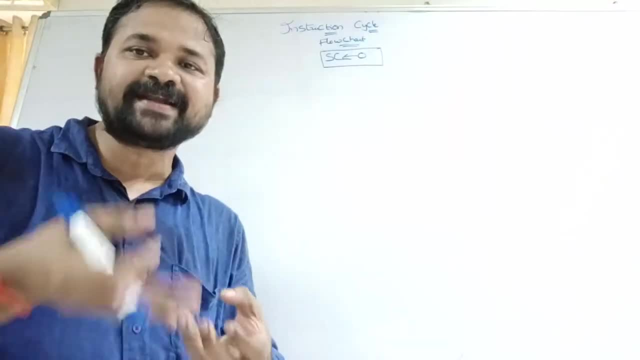 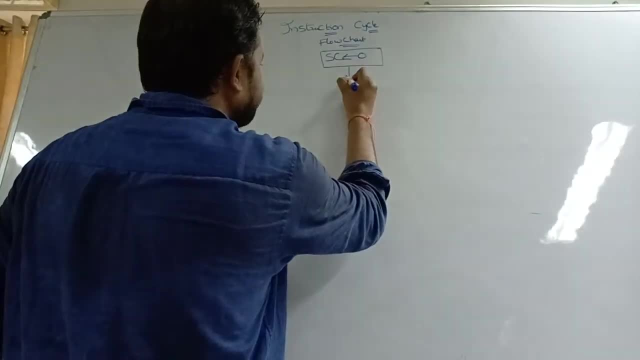 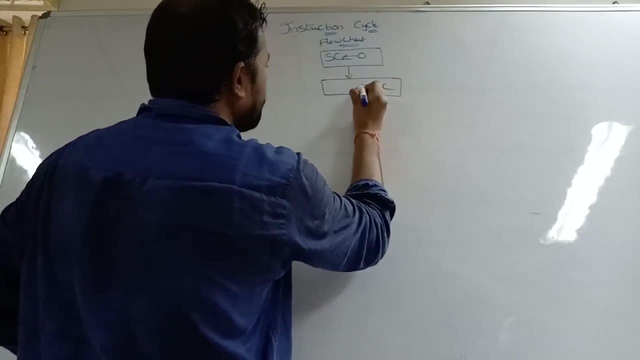 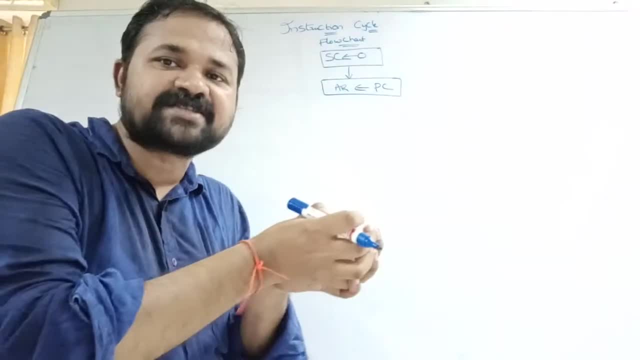 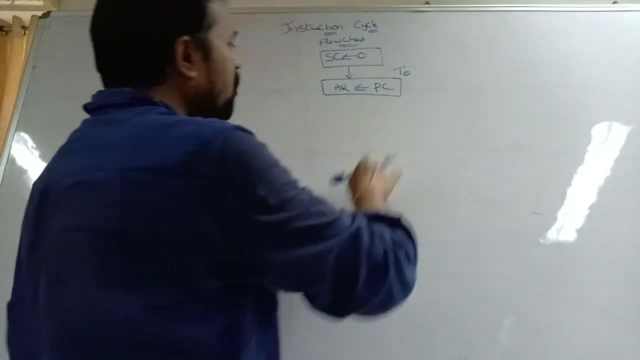 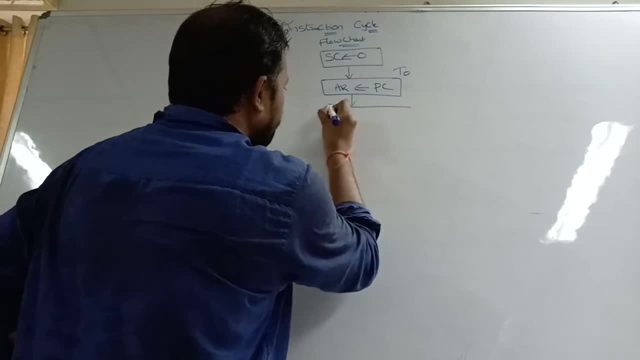 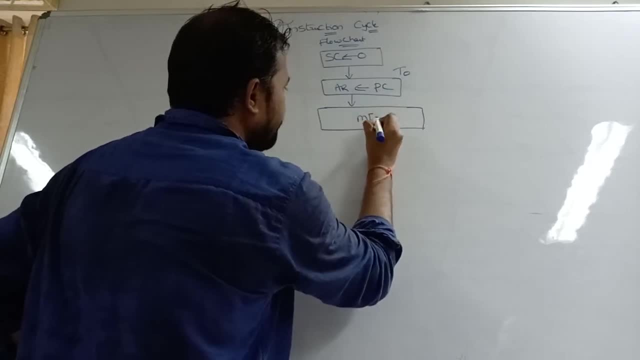 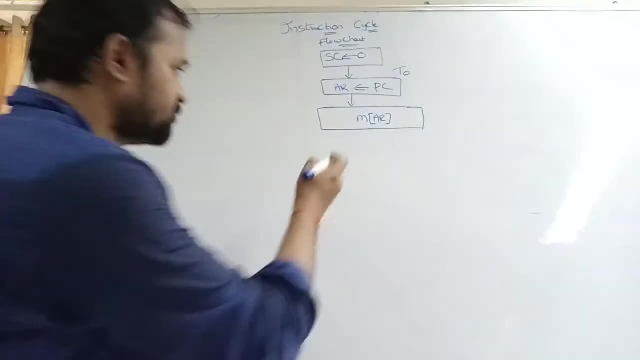 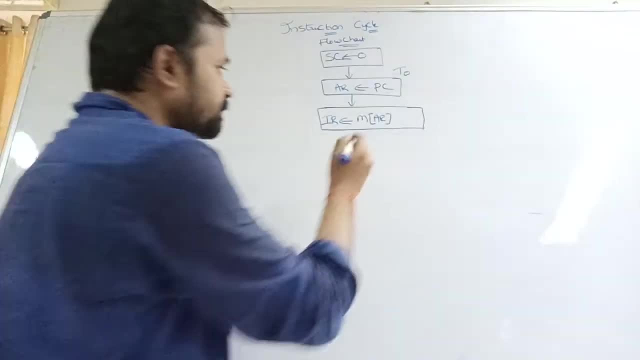 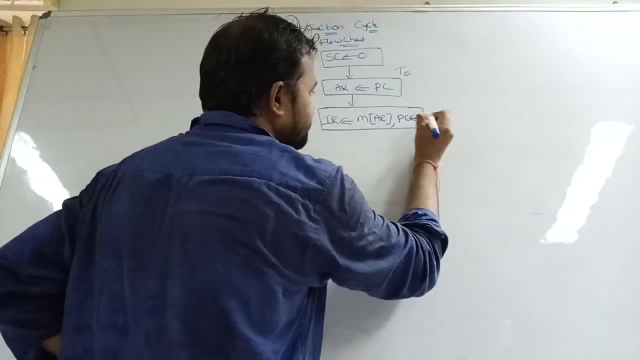 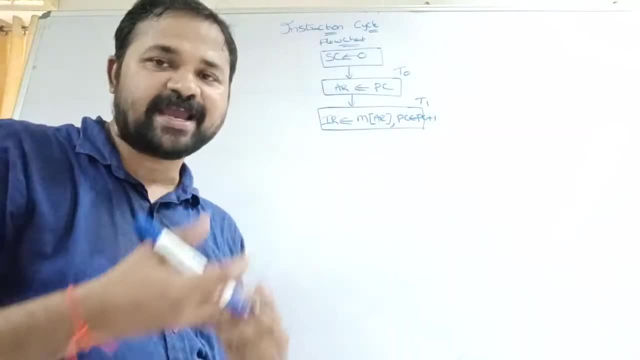 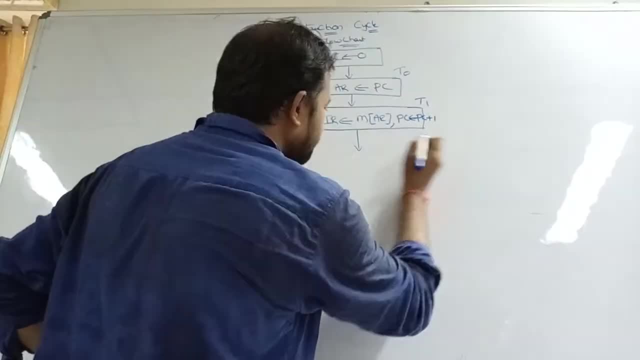 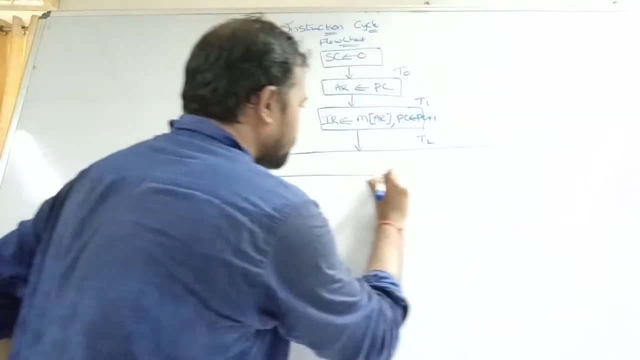 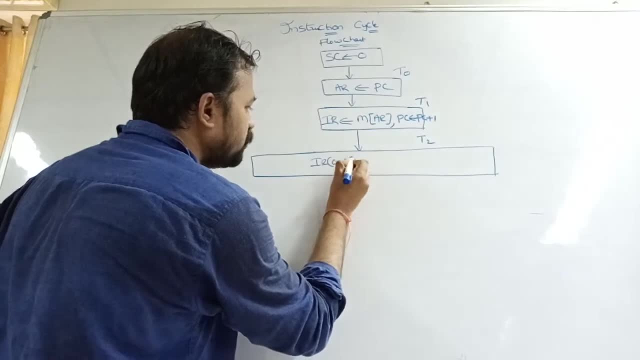 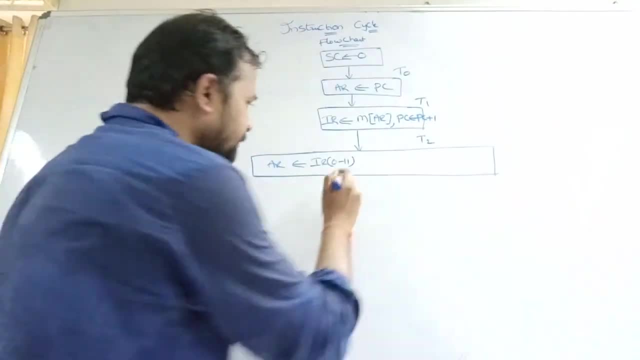 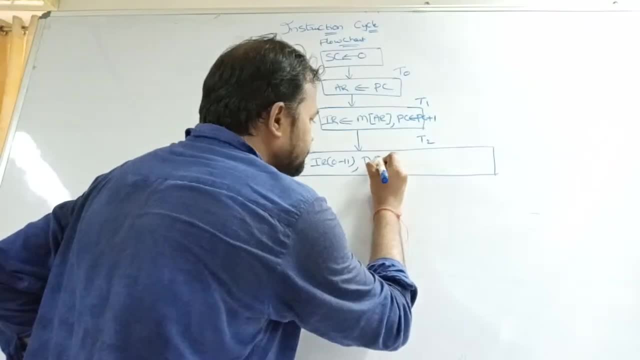 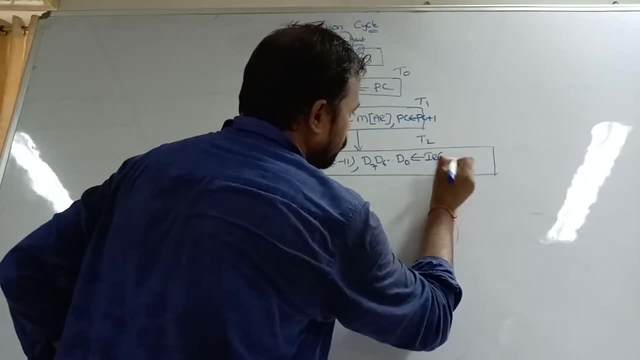 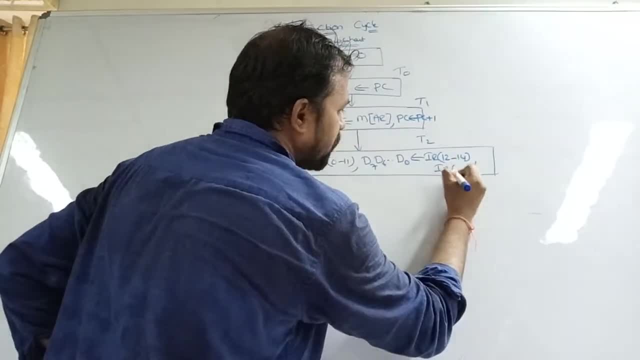 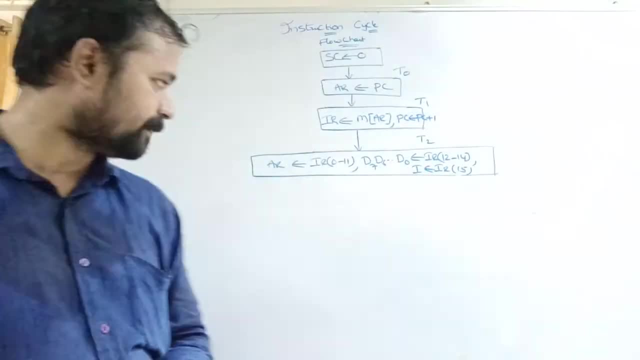 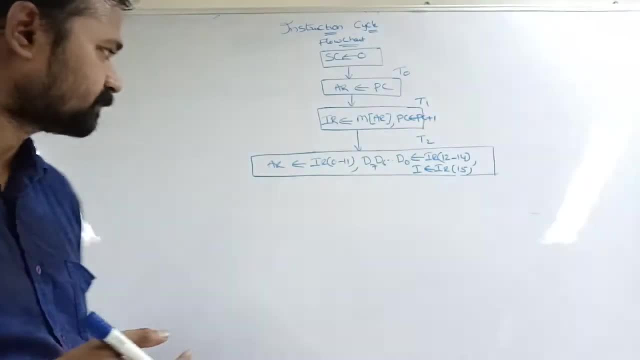 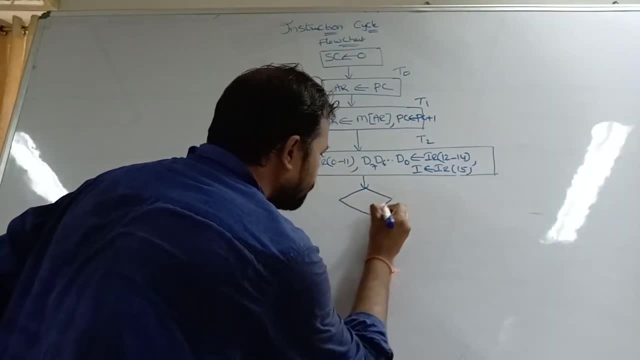 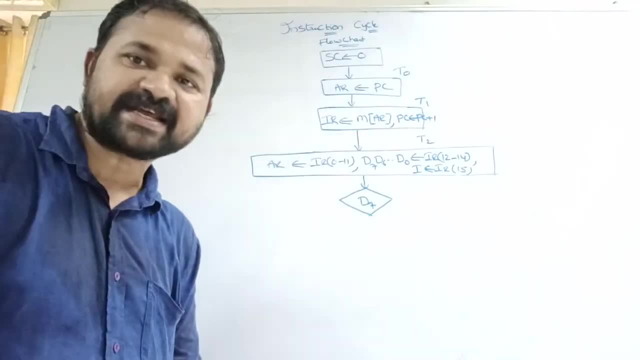 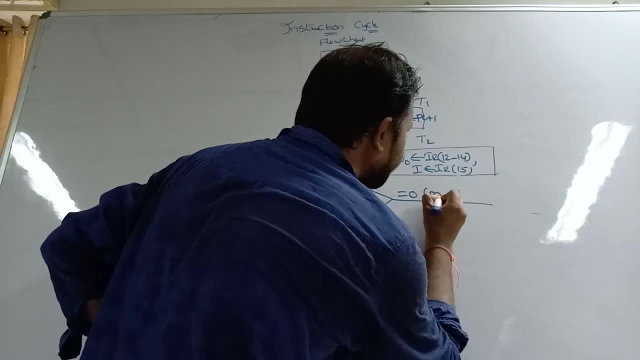 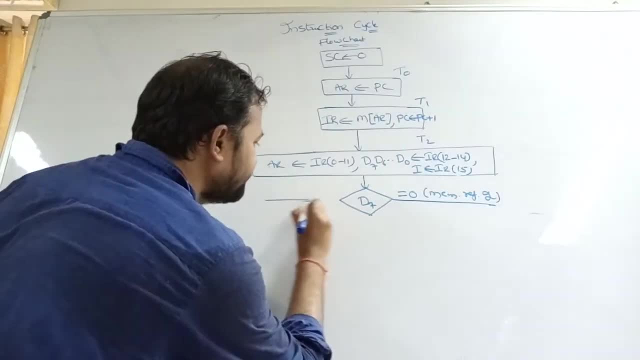 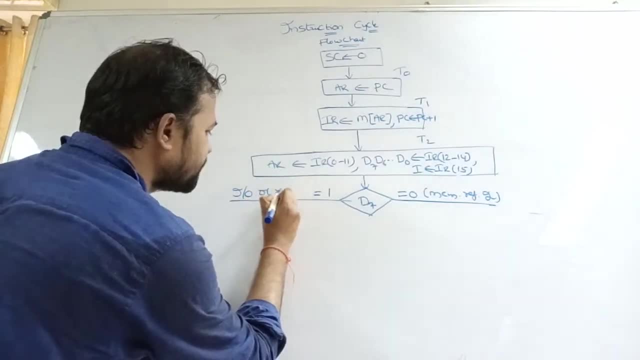 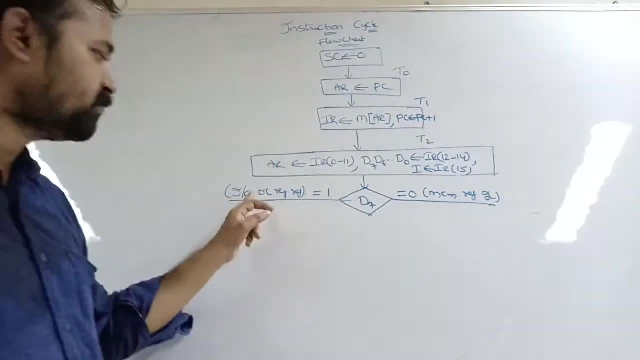 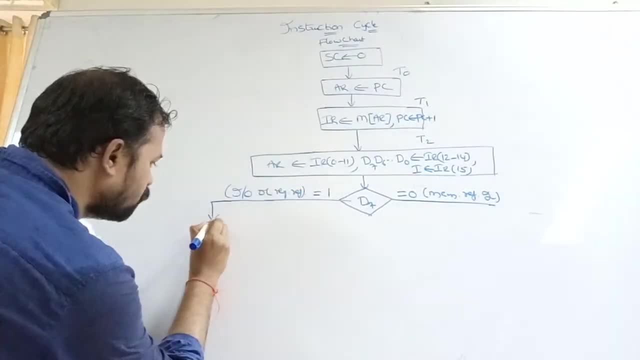 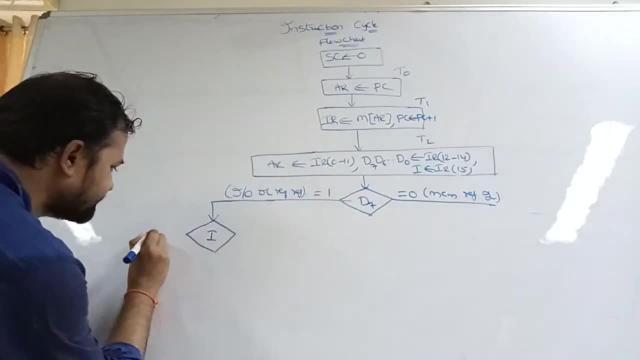 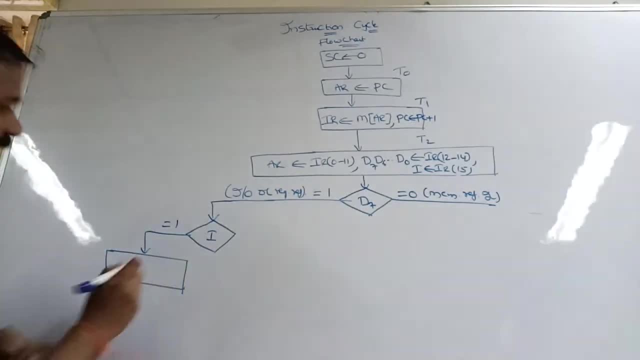 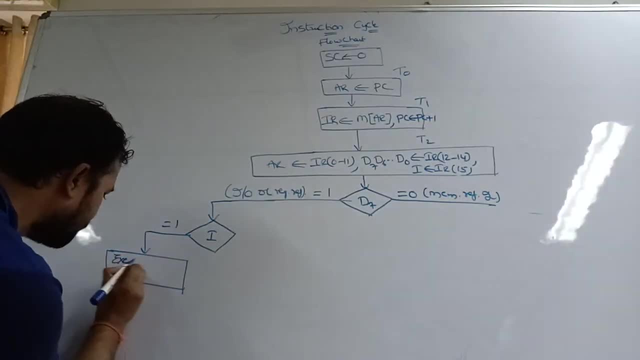 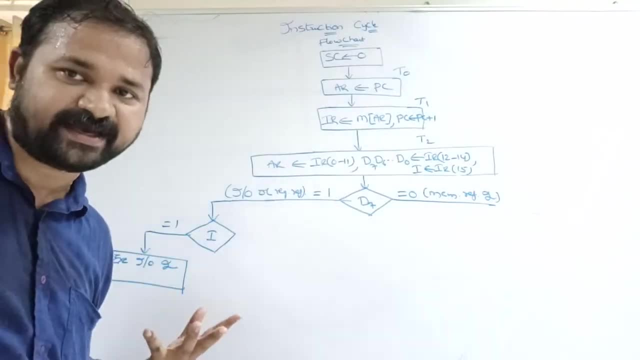 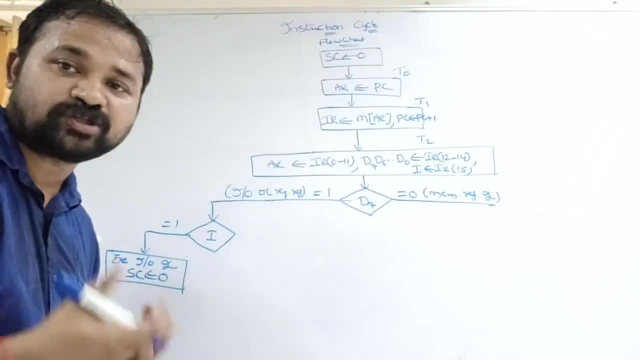 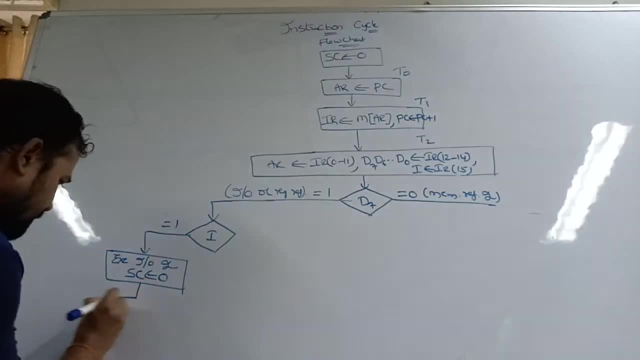 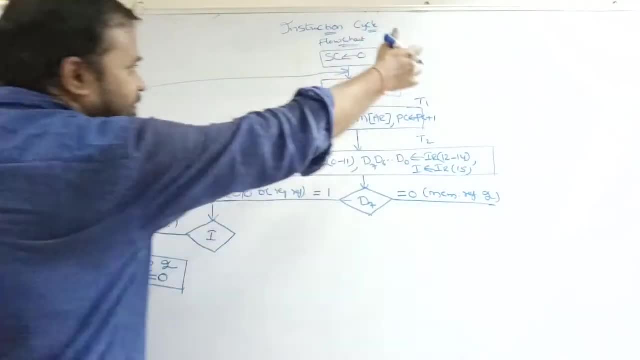 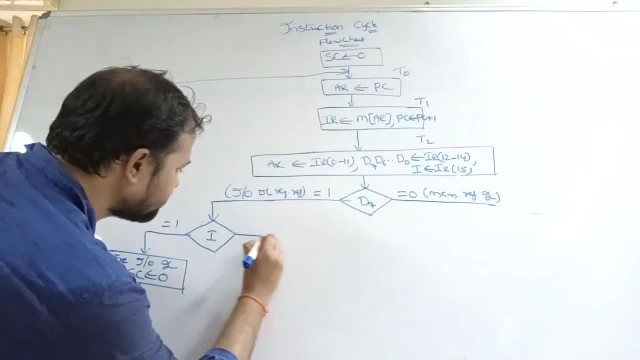 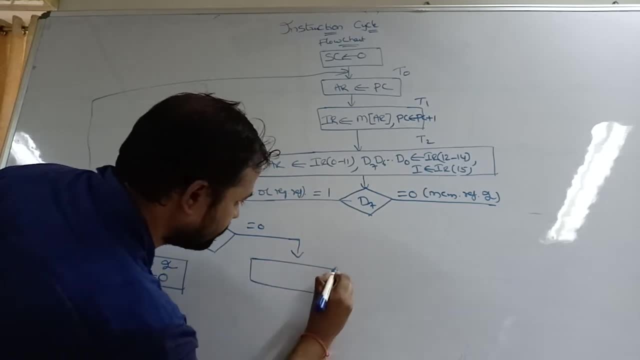 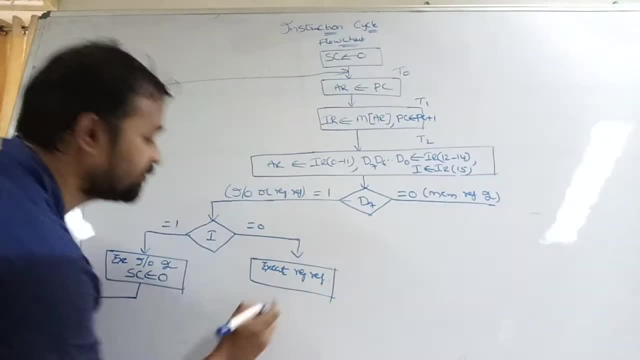 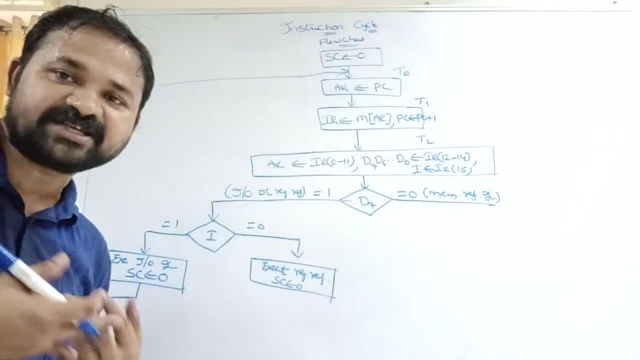 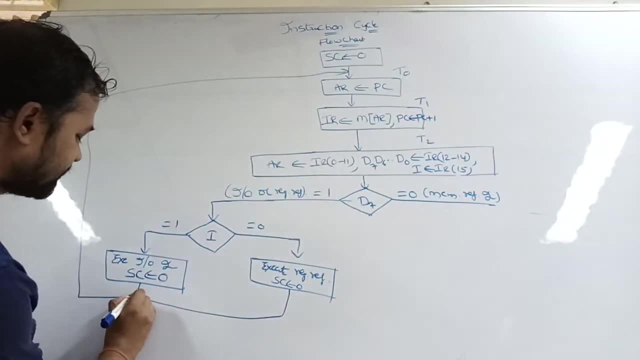 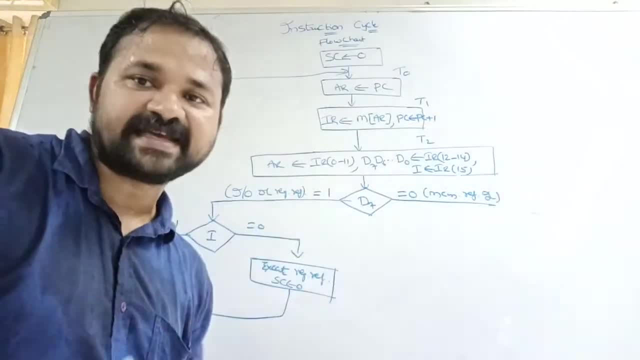 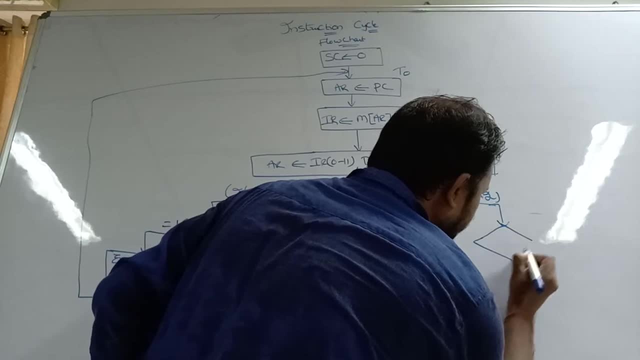 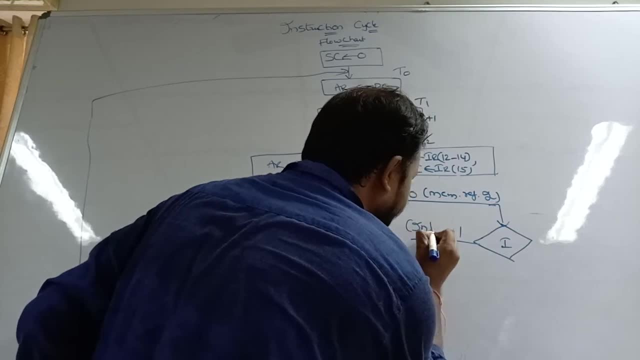 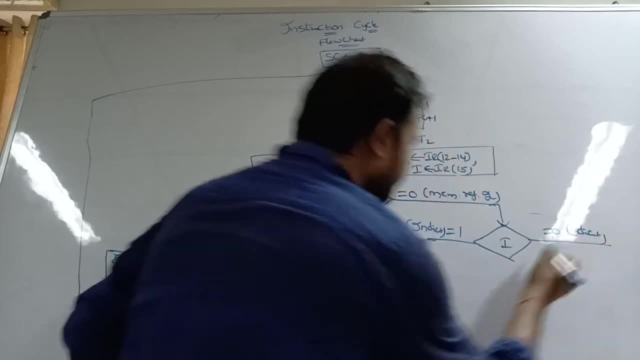 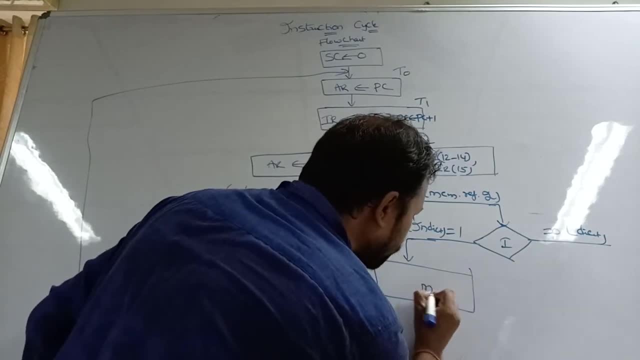 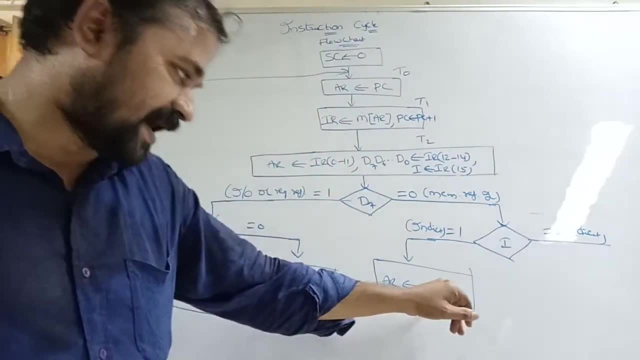 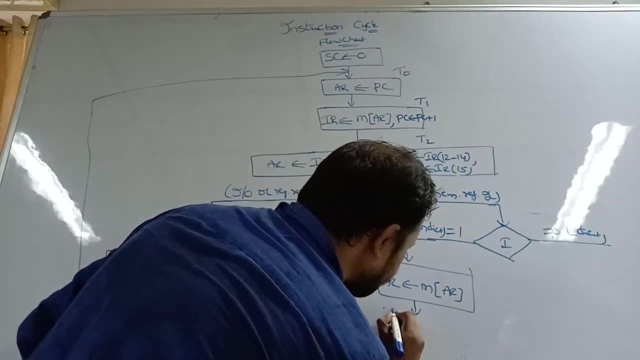 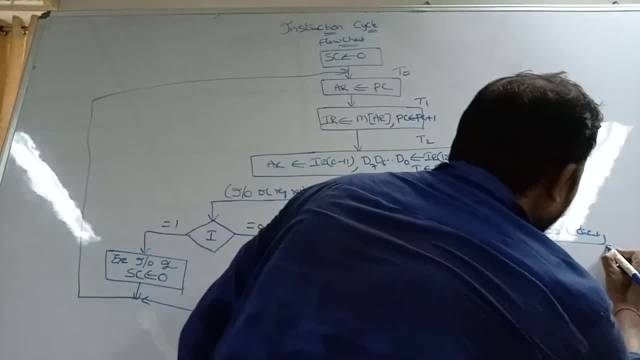 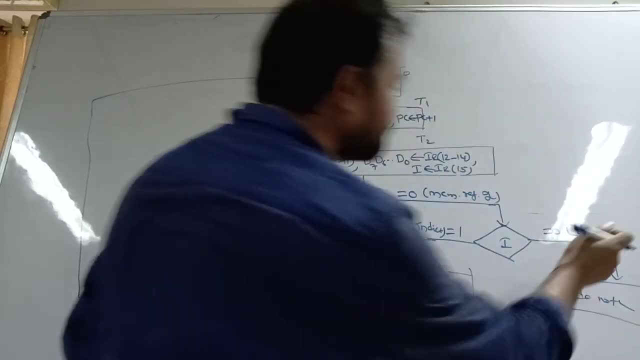 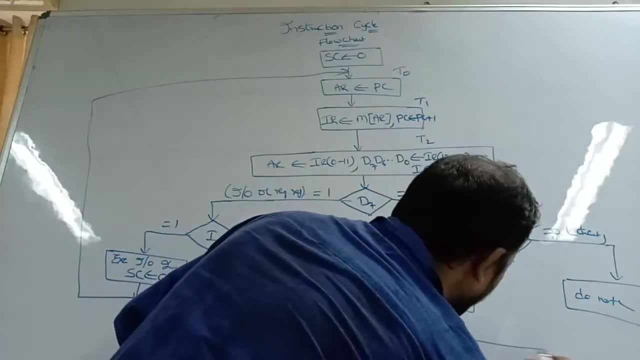 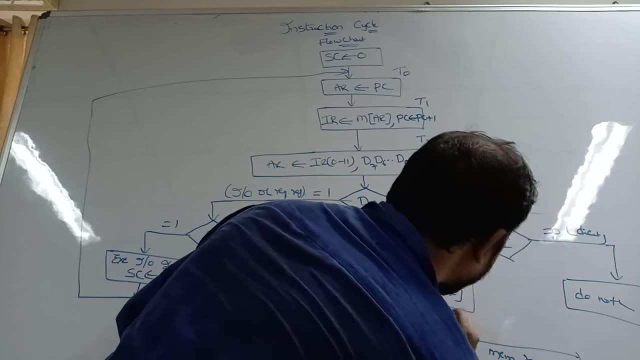